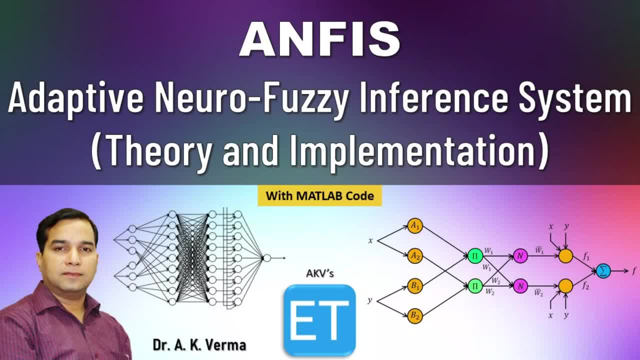 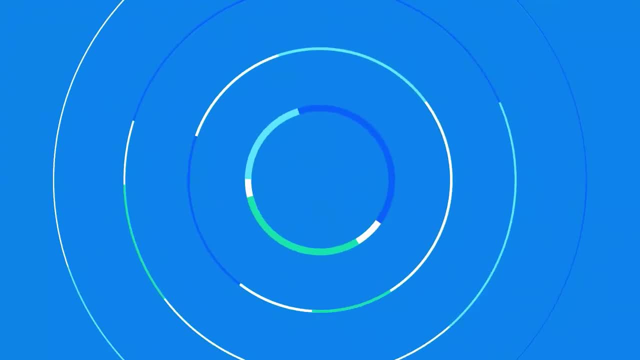 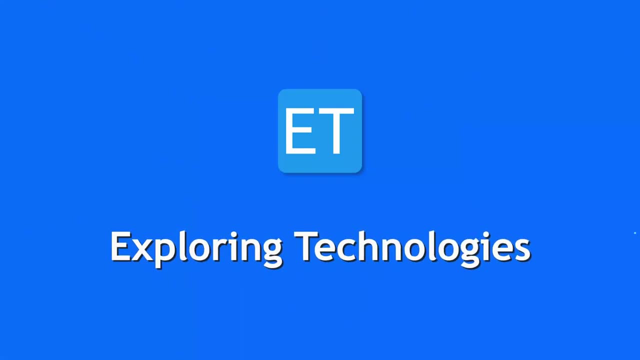 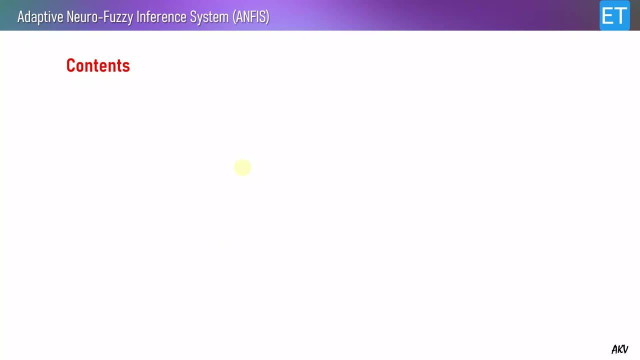 Hello everyone, welcome to Exploring Technologies. In this video I will explain about the Adaptive Neurofuzzy Inference System. In this video I will explain its basic theory and its implementation in the MATLAB. So let me show you the content First. I will 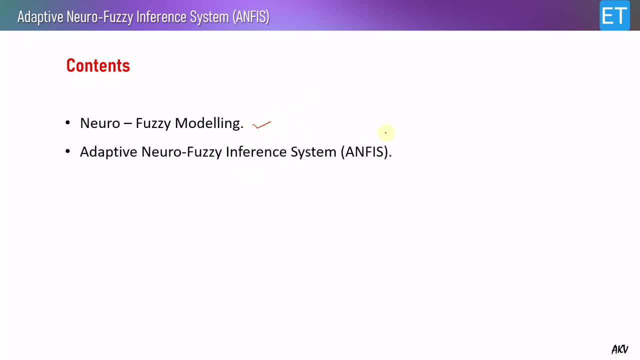 explain what is Neurofuzzy Modeling, Then I will explain Adaptive Neurofuzzy Inference System, Then I will talk about its architecture, Then I will explain its hybrid learning algorithm, Then I will talk about some applications of ANFIS And then I will show you that, how ANFIS can be used as Universal Approximator, And then 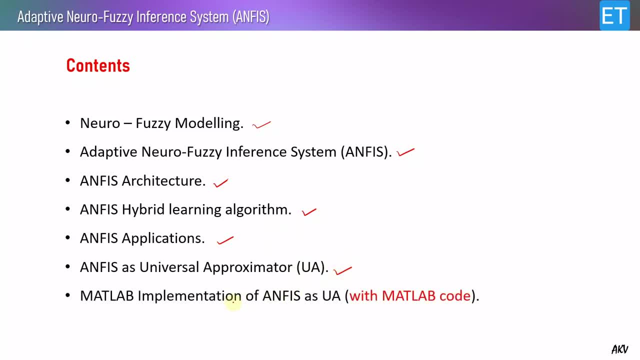 in the last I will explain the MATLAB implementation of ANFIS. For that I will take the example of the Universal Approximator. So I will explain all the MATLAB codes and I will show you the execution of the programs. So that will help you to understand the concept. So now let 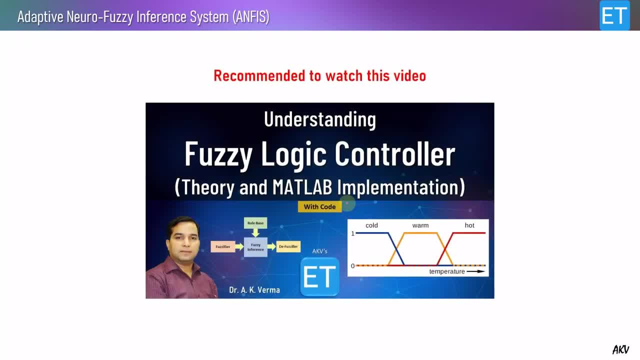 me go ahead, But before going ahead I recommend you to watch my following previous videos. That is about the Fuzzy Logic Controller, where I have explained its theory and I have shown its MATLAB implementation. So the link is given in the description. So if you go, 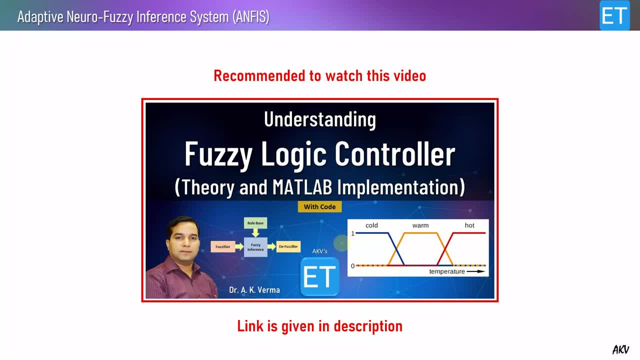 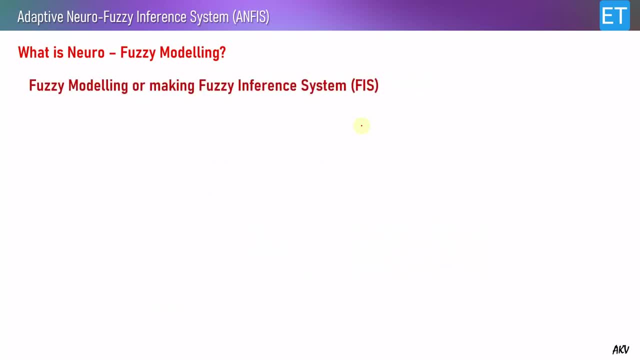 through this video. it will help you to understand this current video. So now let me explain what is the Neurofuzzy Modeling. Before understanding the Neurofuzzy Modeling, let me explain the Fuzzy Modeling and the Neural Network Based Modeling separately, so that you can compare. 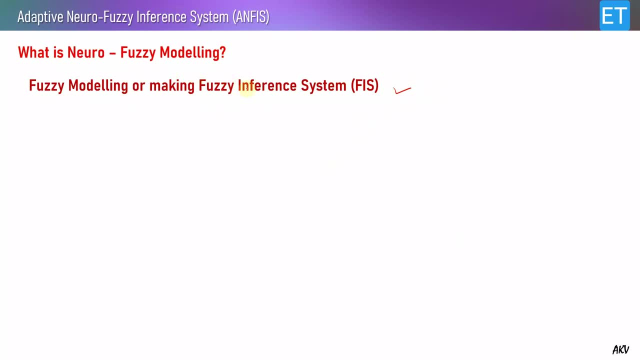 So first I am taking the Fuzzy Modeling or making Fuzzy Inference System. Actually, in many situations it is not possible to obtain the precise mathematical model of system due to its complexity. So in such case of weakness, ill-defined and complex system models, the 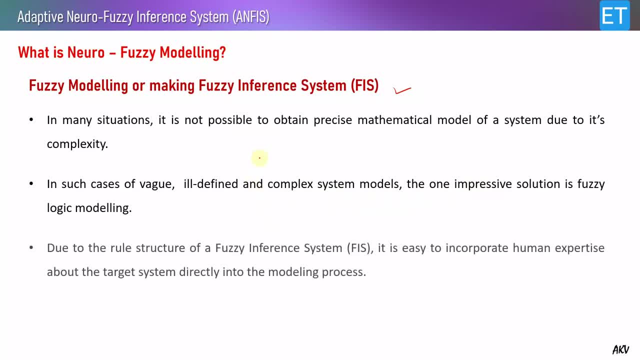 one important solution is Fuzzy Logic Modeling. So due to the rule structure of Fuzzy Inference System, it is easy to incorporate the human expertise about the target system directly into the modeling process. So building a fuzzy system requires both prior knowledge of fuzzy rules, fuzzy sets, etc. 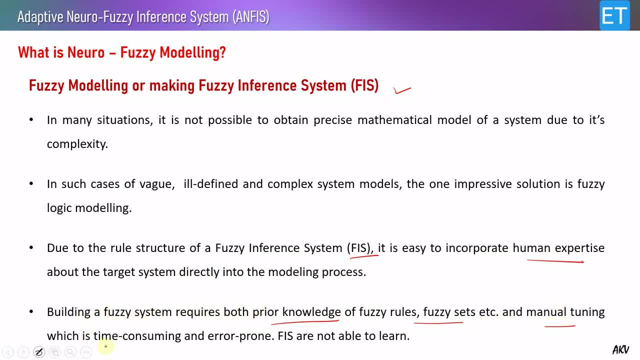 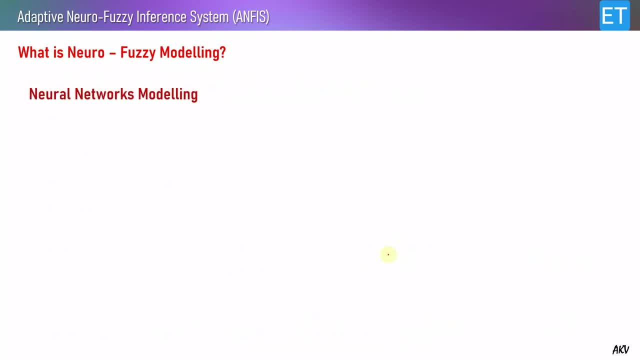 and the manual tuning. That is the drawback, actually So, which is really a time-consuming and error-prone. So FIS are not able to learn. So now let's see what is the Neural Network Based Modeling. So in this approach, the artificial, 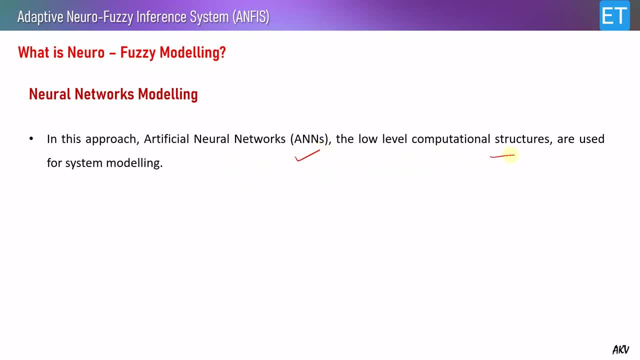 neural networks that are low-level computational structures are used for system modeling. So here neural networks work well. So in the model there are lots of input-output data for target model is available for training. So obviously they have ability to learn. they can change themselves, but ANN cannot handle. 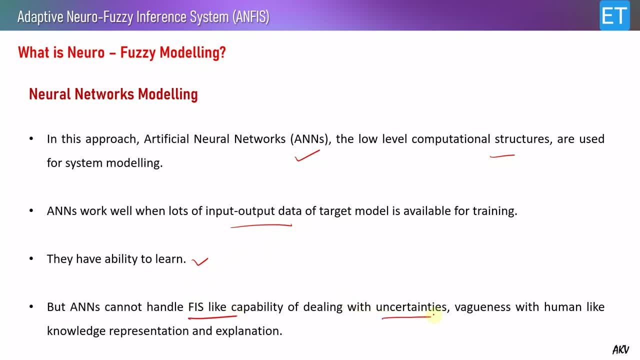 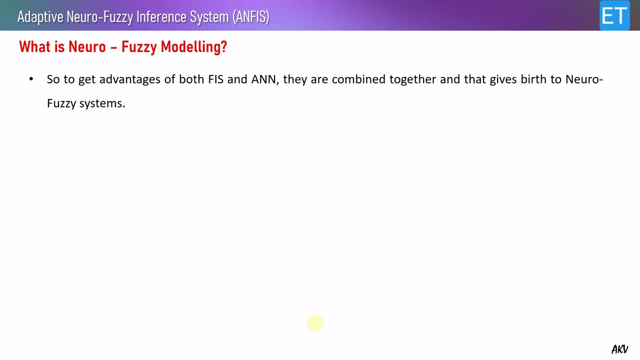 FIS, like capability of dealing with the uncertainties, vagueness and with the human-like knowledge, representation and explanation. So that is a drawback of neural networks. So obviously Fuzzy has some disadvantages and neural networks also have some drawbacks. So now let's go. 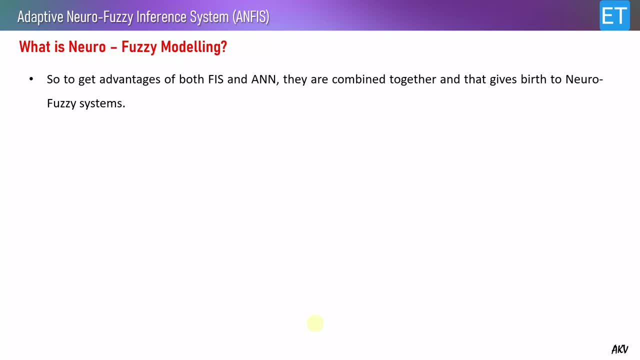 to the next disadvantage. so we are combining them together to exploit their advantages. so to get advantages of both fis and enn, they are combined together and that gives birth to the neuro fuzzy systems. so we can say the neuro fuzzy systems are the fuzzy systems with the learning capability. or we can 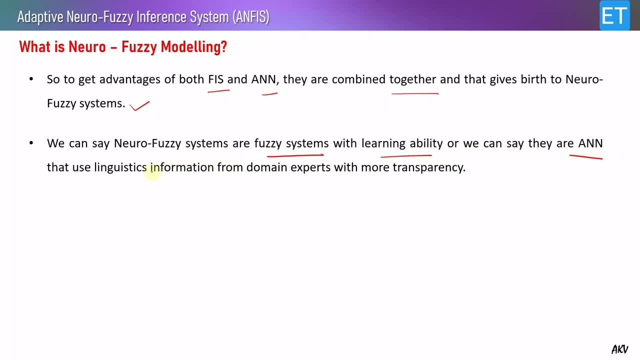 say that they are neural nets that use linguistic information from the domain experts with more transparency. i mean both. both the modeling approaches are taking advantages of both approaches. so we have several combination schemes. i mean how to combine fis and enn together. the first one is a cooperative neuro fuzzy systems, concurrent neuro fuzzy systems and the hybrid. 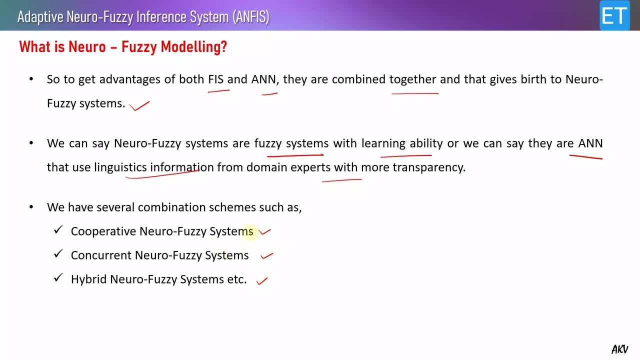 approach in cooperative neuro fuzzy systems. actually neural nets are used to fine-tune the fuzzy systems. the neural nets are only used for tuning purpose- okay, after that they are removed and only the fuzzy systems then works. but in concurrent neuro fuzzy systems both work together and hybrid is. 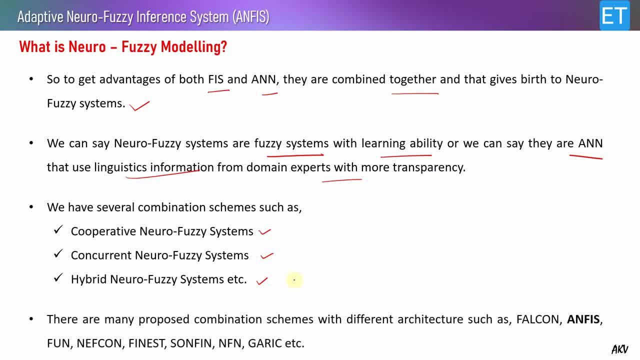 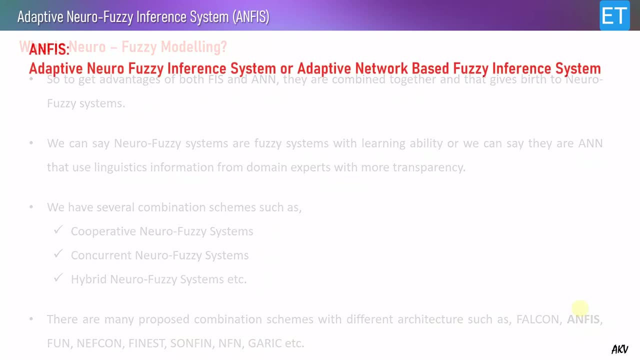 also a similar approach. so there are many proposed combination schemes with different architectures, such as falcon and face, fun, nefcon, etc. so in this video i'm concentrating only on and face. so let's see what is this. and face and face is known as the adaptive neuro fuzzy inference system. 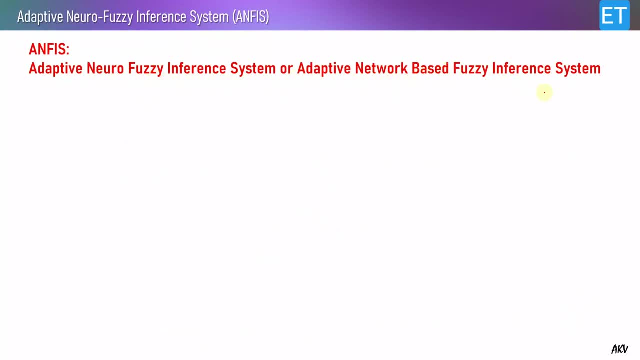 or adaptive network based fuzzy inference system. so and phase is actually the neuro fuzzy system that uses five layer network with supervised learning. it was first proposed by the roger chang and son in 1994. the link of the research paper is given in the description. you can refer. 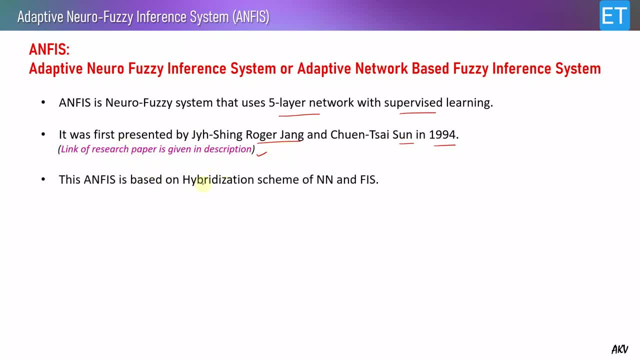 that or you can search on the google. so this and phase is based on the hybridization scheme of an nfis. that is just i have explained in the previous slide, the third approach. so it has become very popular and has been used in number of applications since then. so it is simple and very efficient when number of inputs are less. 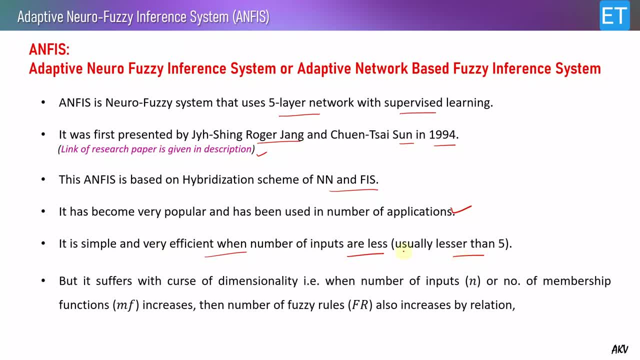 usually lesser than five. but it suffers with the curse of dimensionality. it means when the number of inputs- all the number of membership functions per input- increase, then the number of fuzzy rules also increase by this relationship. so fuzzy rules, the number of fuzzy rules, are equal to the number of membership functions. 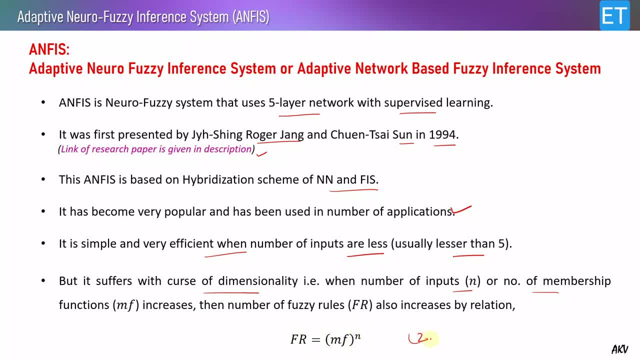 power. number of inputs. so if you have, let's say, two membership functions for each input and the number of inputs, let's say, are 10, then there will be 10024 fuzzy rules. okay, so it demands a huge computational efforts. so the computational complexity is the main drawback of the n-phase when the number of inputs are large. okay, now let me show you the. 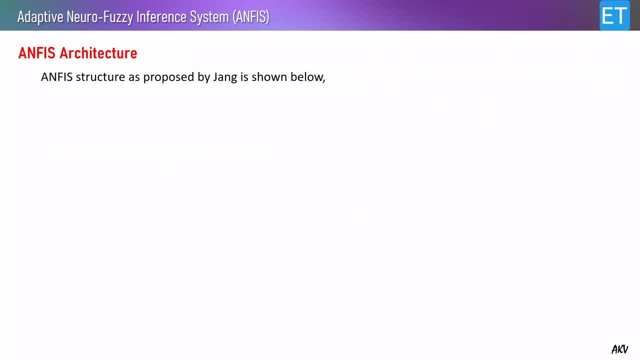 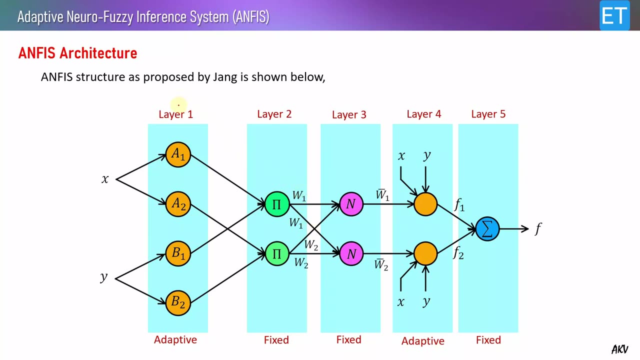 structure of the n-phase uh that was proposed by the zhang. so this is the network structure which has the five layers: layer one, layer two, three and four uh. in the layer one we have the, actually the membership functions. so for the two input, this uh network shown here is for two inputs. 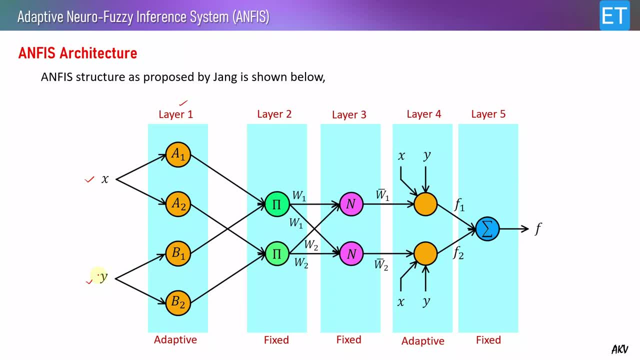 uh, if the inputs are uh different- i mean more than two- it's a structure will change and we have two membership functions for each input. i mean a1 and a2 for x, b1 and b2 for y. so if i increase the number of membership functions also also uh, its uh appearance will. 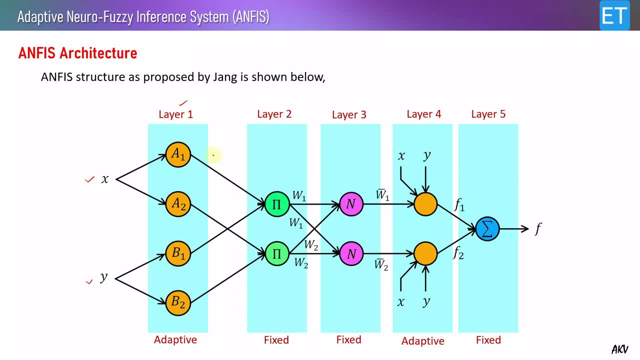 change. so this is the case of two inputs and two membership functions for each input. so the layer one is actually adaptive layer. that means the values of uh a1, a2, b1, b2 between the inputs change during the training. in the layer 2 it is a fixed layer. the nodes are: 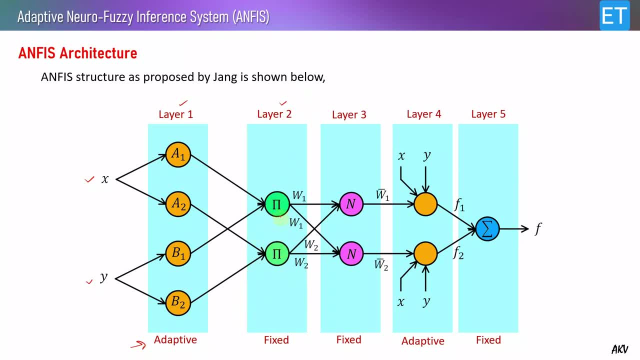 fixed, so they have the multiplication operation. so the output w1 of this node is obtained by multiplying these two incoming signals. and layer 3 is a normalization layer, that's why represented by the N, so here weights are normalized. later I will show you that, how normalization is obtained, and 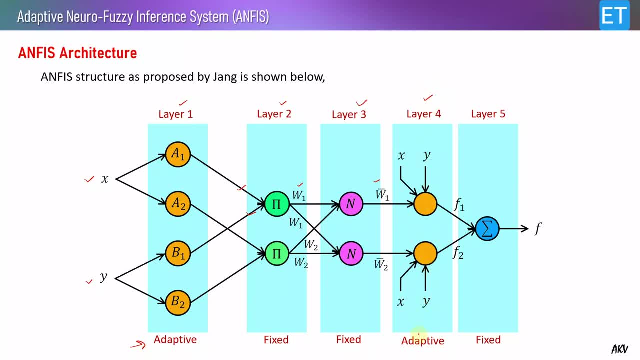 the layer 4 is again the adaptive layer. here, during the training, the values are updated. and in the layer 5 we have a single node which is a summation node. so output F depends on the, simply the summation of all incoming signals to this node. so now let me explain the function of each layer in detail, one by 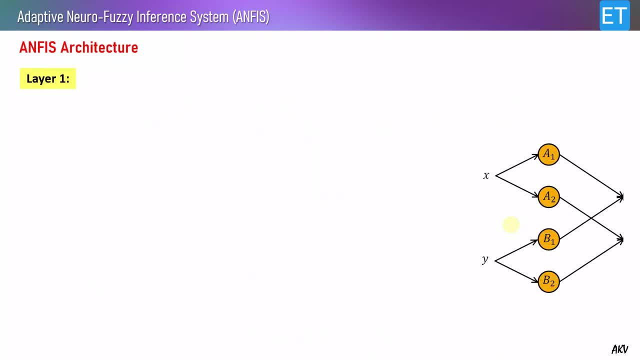 one. so first the layer one. so this is the part of the layer which we have just seen in the previous slide. so, as I said, for the two inputs, X and y, I have the two membership functions, a 1 and a 2 for x, b 1 and b 2 for y. so these are the 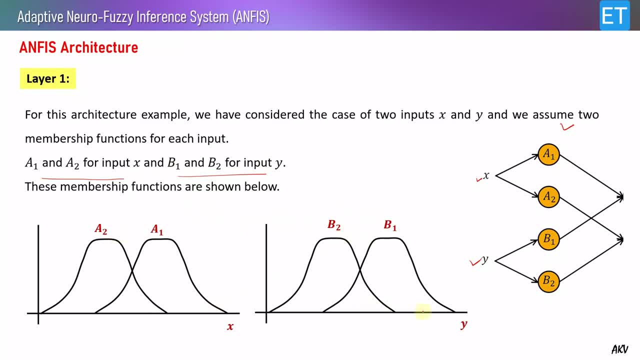 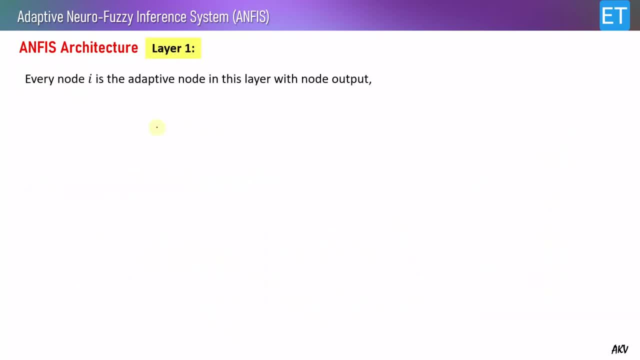 membership functions: a 1, a 2, b 1 and b 2 for x and y respectively. so these are the Bell functions, so the, as I said, the node, every node in this layer is adaptive and the output is given by these two equations. so the output is given by these two equations. so the output is given by the. 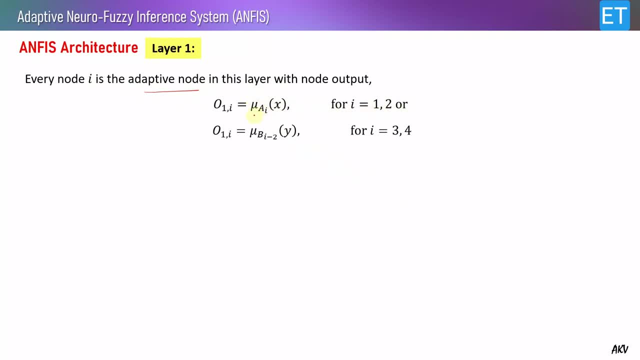 So for i equal to 1 to 2, I get mu A1x and mu A2x, like this: mu A1x and mu A2x. And for i equal to 3 and 4, I will get mu B1y and mu B2y. 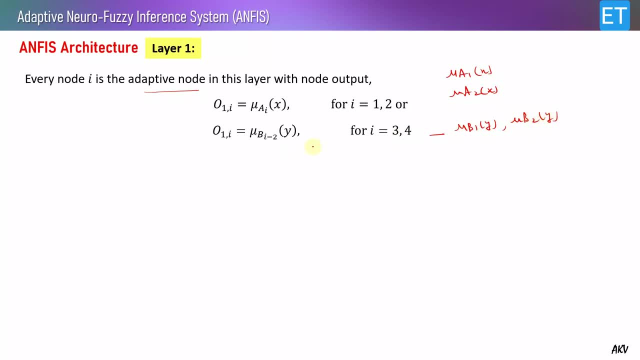 So I get four values for two inputs- x and y. So that is actually the fuzzification. So for two crisp values- input values x and y- I get these four fuzzy values. So this is the operation. you can clearly understand from this figure that for a particular given value of x, I get these two fuzzified values. 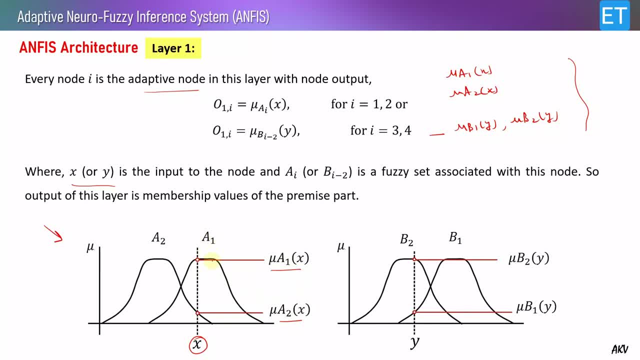 You can say that the x cuts the membership function at this point, So I get mu A1x. and it cuts the membership function A2 at this point, so I get mu A2.. Similarly, I get mu B1 and mu B2y for the given value of y. 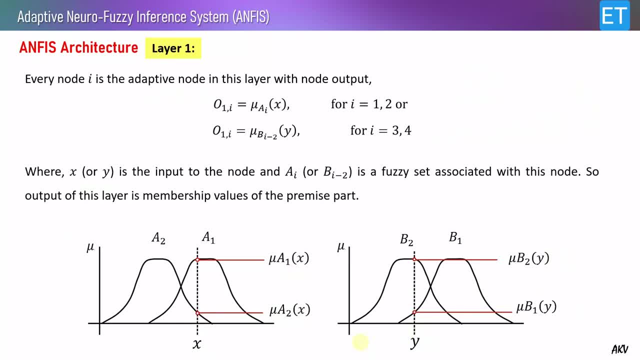 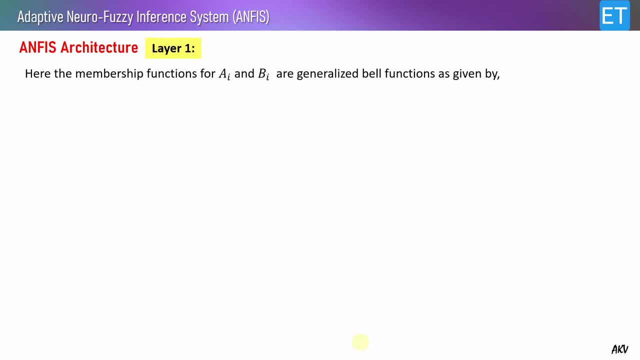 So this is how the fuzzification takes place. And now, as I said, that membership functions are actually the bell functions, So that is the expression which is governing the shape of the membership functions. So here are the parameters: I, B, I and C: I. 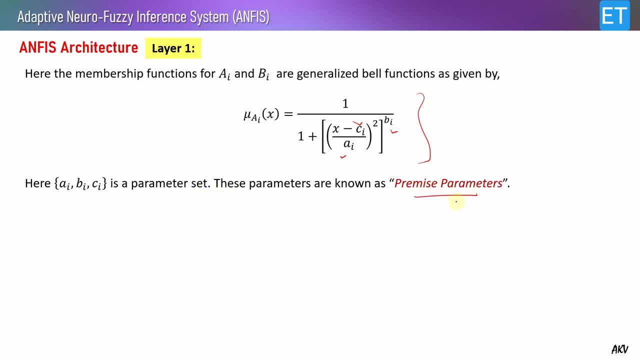 So these parameters are known as the premise parameters. So these parameters are updated during the training process. Later we will see that how they are updated. Now let's come to the layer 2.. So in this layer every node is a fixed node, as I said, and the level adds pi. 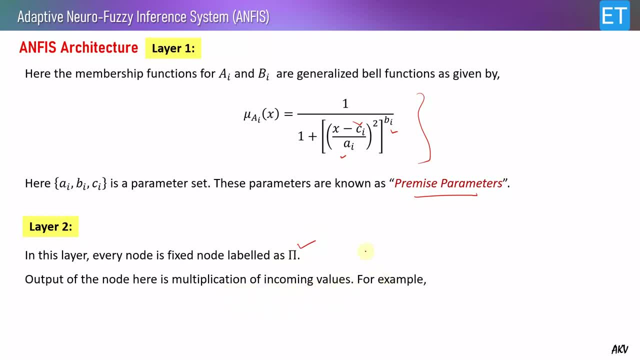 The output of the node here is a multiplication of all the incoming values, So obviously the output, The second layer node, is wi, represented by the wi, where output is simply the multiplication of these two fuzzy values, mu, Aix and mu By Okay. 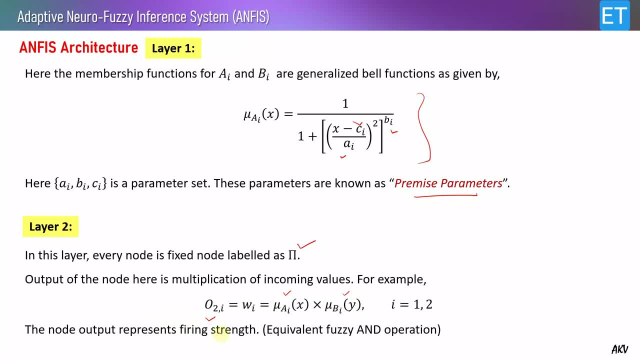 So actually the node output represents the firing strength And this operation is equivalent to the fuzzy end operation. So it means I will perform the minimum operation. So later I will tell you that what is equivalent to this mu. So I will tell you that what is equivalent to this mu. 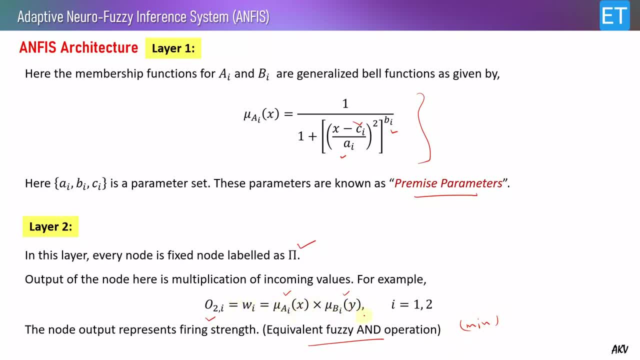 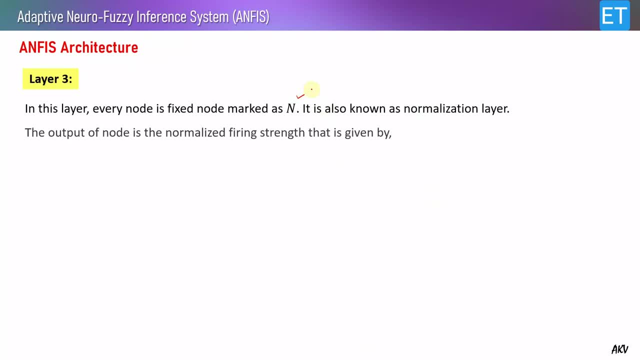 So I will tell you that what is equivalent to this mu? Therefore, in order to define mu, I have to所 luce to that same equation. mu Aix into mu By, like this: And in layer 3, this is the normalization layer marked by N. 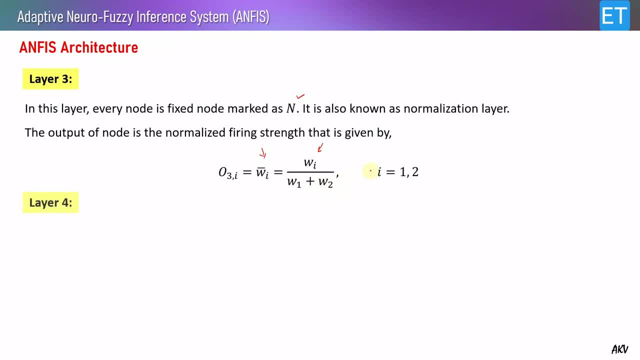 The normalization is done by this equation, so that is a normalization of the firing strength. and in layer 4, which is again the adaptive layer, the output of the node in this layer is given by this equation, that is wi bar, which is obtained from the layer 3 multiplied with fi. so what is fi? this is fi. 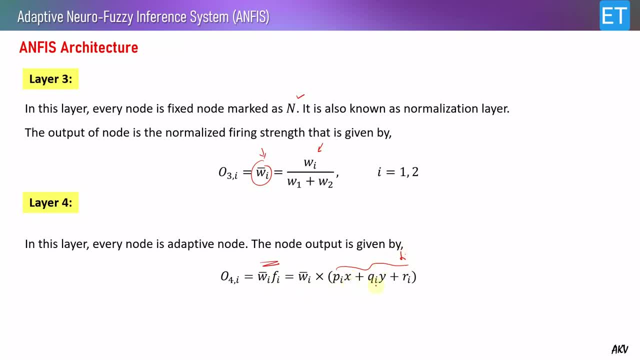 so fi is given by pi x plus qy, y plus ri. here x and y are input, while pi qi ri are the parameters. so these parameters are known as the consequent parameters and they are updated during the training process. okay, and now layer 5. so this is a final single node which is labeled as a sigma. 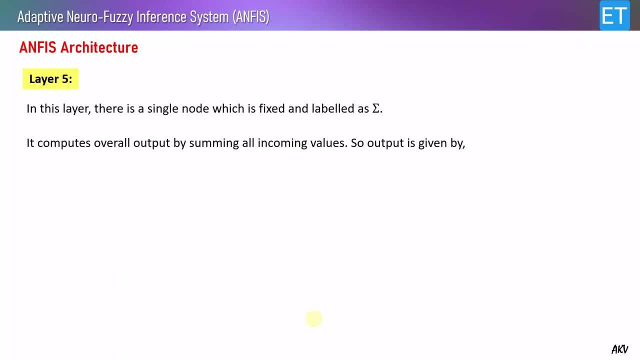 and its function is obviously the sum sigma, and its function is obviously the sum sigma and its function is obviously the sum summation of all incoming values. so this is how i get the total output and this is how my neural networks, as exactly the sogenan type fuzzy inference system. so this structure is not unique. 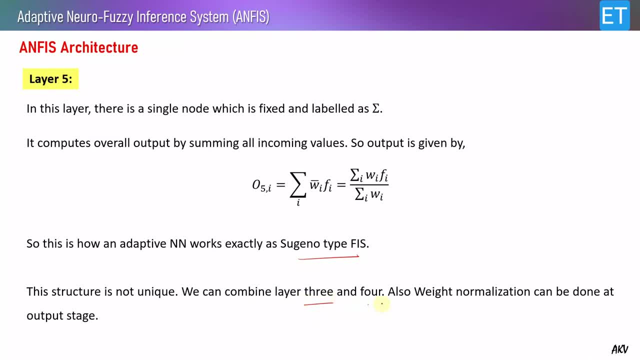 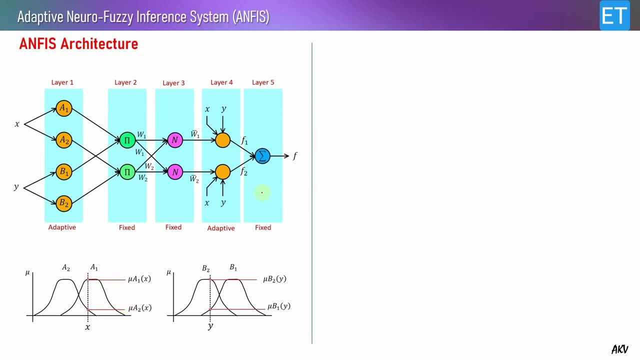 we can combine the layer 3 and layer 4. also, the weight normalization can be done at the output stages. so there may be some change in the network. and now let me summarize all those mathematical operations here. so for input x and input y i get the four fuzzy values, as i said. 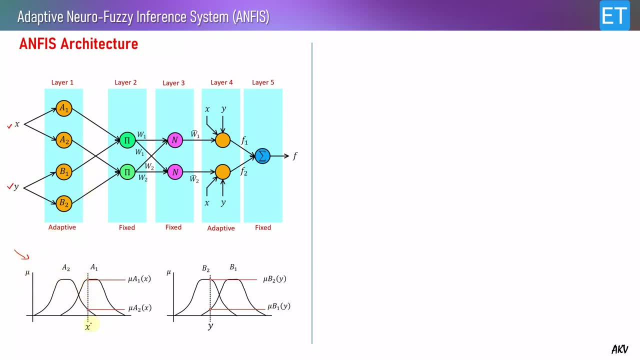 so from this figure for the particular given value of x, i get mu a1 x and mu a2 x. so here i get mu a1 x and here i get mu a2 x. at this point i get mu b one y, and here i get mu b two y. okay, so that is a. 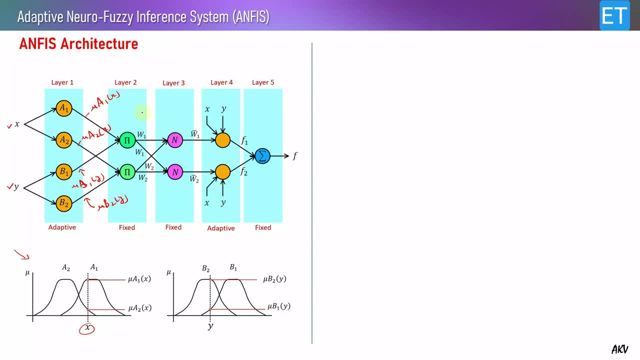 fuzzification. and now in the layer two, uh, i get the w1. so w1 is the output of the node and that is simply multiplication of the two incoming fuzzy values. so mu a1 x multiplied with, uh, mu b1 y, mu b1 y- okay. and similarly w2 equal to w2, that is, mu a2 x, mu a2 x multiplied with mu b2 y, okay. so now, uh, what? 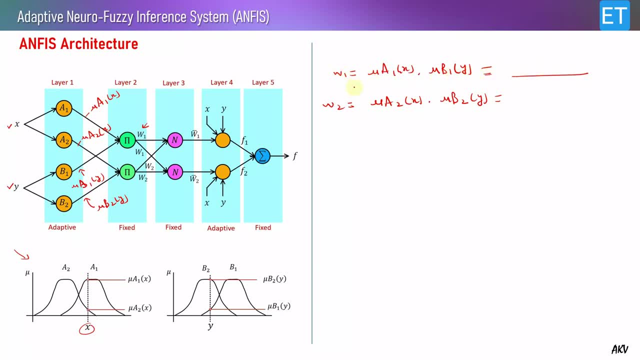 i should write here uh, as equivalent to w1, as i said in the previous slide, that this operation is the end operation. okay, so i will take the minimum out of these two. so just go to this figure and compare mu a1 x and mu b1 y. so mu a1 x is this, and 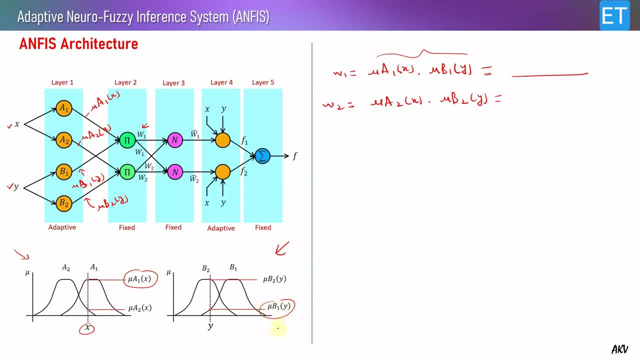 mu b1 y. is this? so which one is minimum? obviously mu b1 y. so my output is mu b1 y. okay, for w2 i have to compare mu a2 x, mu a2 x and mu b2 y. so which one is minimum? obviously mu a2 x. so my output is: 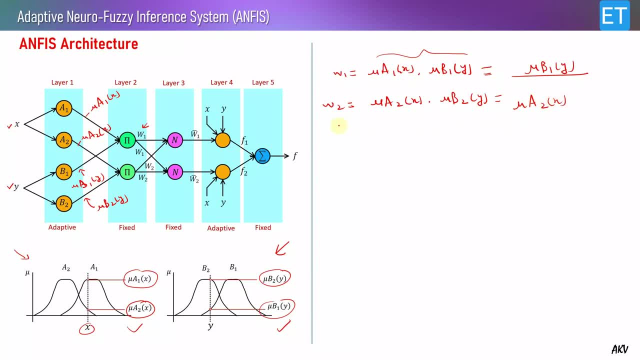 mu A2, mu A2 x. so that is the expression of w1 and w2, now the normalization. so w1 bar is w1 upon w1 plus w2. so w1 is a mu b1 y upon mu A2x, uh, plus mu b1 x and mu b2y. 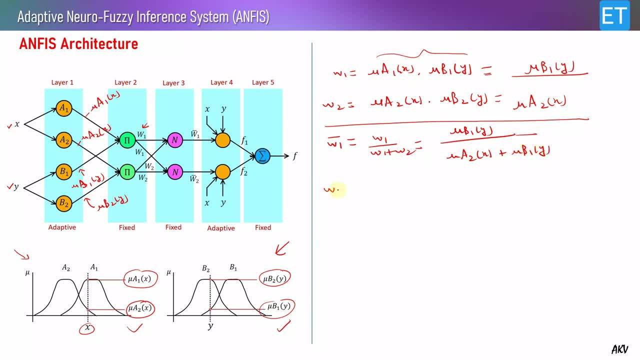 y. okay. similarly i can write for w2 bar, so that is w2 upon w1 plus w2, so that is mu a to x upon mu a to x plus mu b1 y. okay. so these are the expressions for w1 bar and w2 bar. 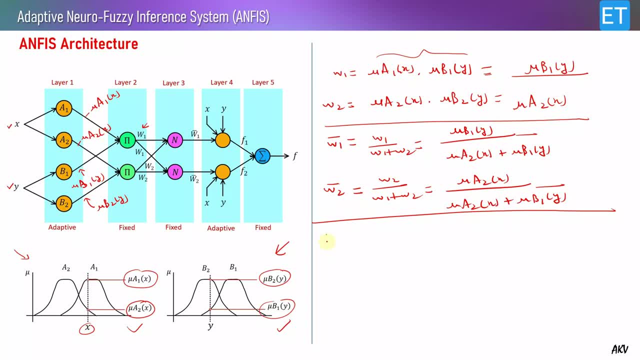 now i can write expression for f1 that is the output of the layer 4. so f1 is simply w1 bar into p1, x plus q1, y plus r1, and f2 is w2 bar into p2, x plus q2, y plus r2. 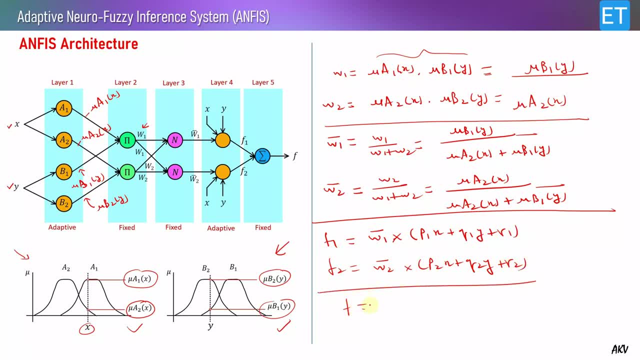 okay, and the output is summation of these two, so that is simply f1 plus f2. so from this equation and this equation, if you sum these outputs f1 and f2, you will get output. so this is the actually overall summary of the mathematical operations in this neural net. 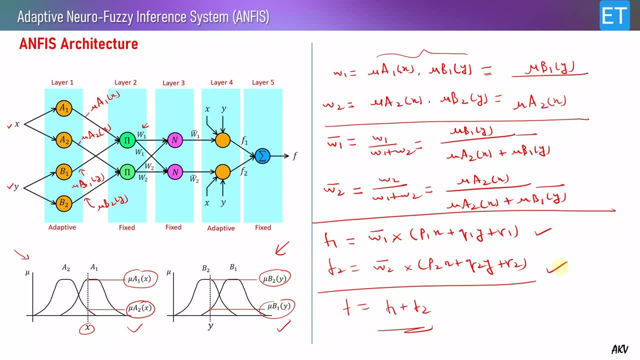 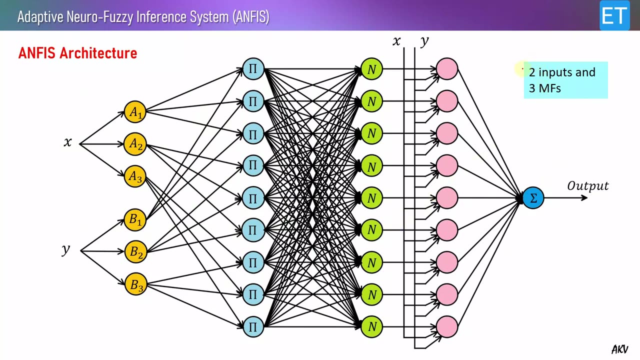 and now let's see the architecture with a more complexity, where the number of members of functions are increased. so this is one example where the complexity has increased. so here we have the two inputs again, but the number of membership functions are increased. so instead of two, now i have three membership functions. okay, so when the membership functions 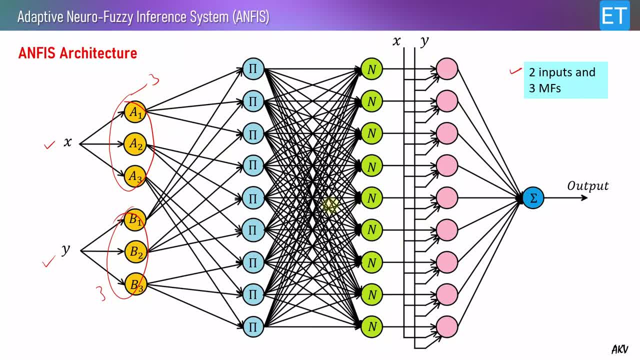 are increased. you can see the complexity has increased. so how many rules are there? so fuzzy rules are membership functions, power, numbers of input. we have the number of inputs. i mean three power two, so that is nine. so obviously we have the nine rules: one, two, three, four, five, six, seven, eight and nine fuzzy rules. 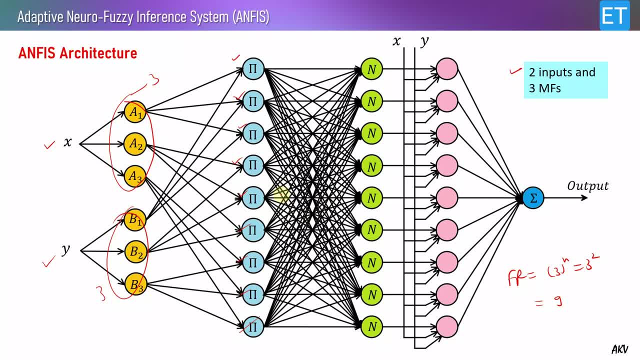 so this is uh just to show you the complexity uh of the network. uh, here is still. the inputs are two. if i increase the number of inputs also, then you just can imagine the complexity of this network. so that is the drawing of this network. so let's just make a number of inputs now to count the input ups and downs. 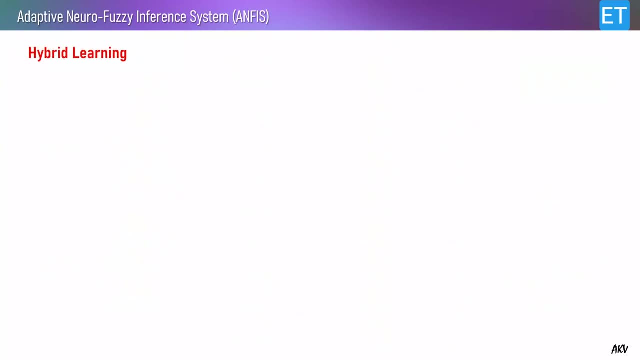 of Enphase. so now let me explain the hybrid learning. so what happens during the training actually? so here both side parameters, the premise parameters, and the concept, the consequent parameters, are modified, as I said. so premise parameters are at the input side, I mean those a, i, b, i and c, i which are actually governing the shape of the membership functions, while 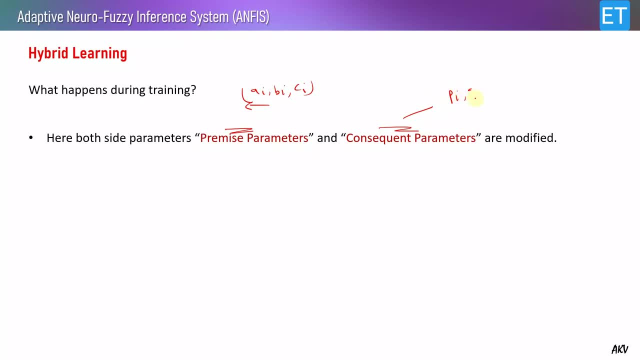 the consequent parameters were p i, q, i and r i. okay, so in forward pass, the premise parameters are fixed. okay, so these parameters are fixed while the consequent parameters are updated using LSE least square estimate. and in backward pass, the premise parameters are updated while 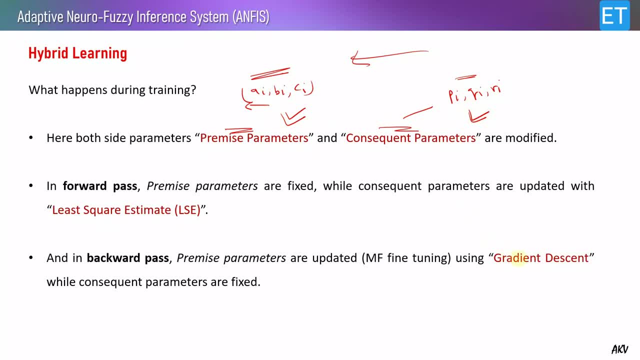 the consequent parameters are fixed and this updation is using the gradient descent that is known as the membership function- fine tuning, as I said, because a, i, b, i, c, i are governing the shape of the membership functions, so during the backward pass they are fine tuned. so this is the actually the hybrid learning approach. so followings are some applications. 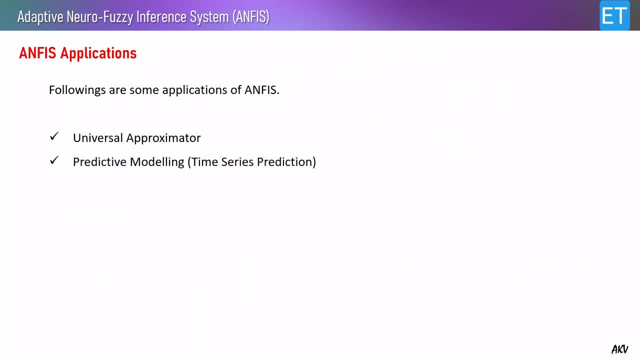 of Enphase. one is the universal approximator predictive modeling, that is, a time series prediction. hopefully I will explain this in the next video. the controller design pattern: Georg M Sprinkleall. this algorithm is also used in the rar to represent the optimization of氧ут and the. 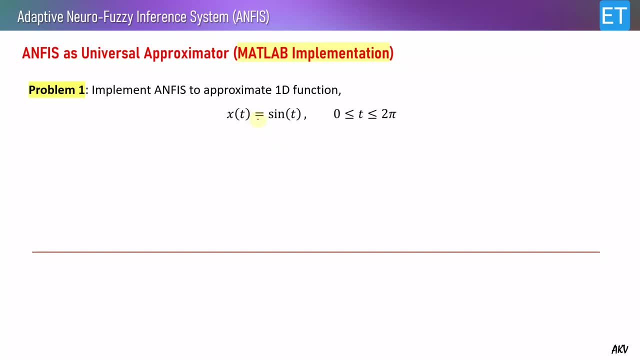 communication simulation that is designed to predict the 함dt-1M mange commands r m phase to behave like a sine function. and in the second example I will implement this two-dimensional sinc function, sinc function. okay. so my n phase model will behave like this sinc function. so what are the steps in MATLAB I have to use? 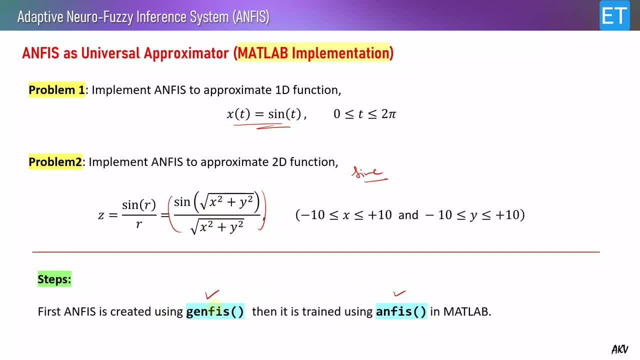 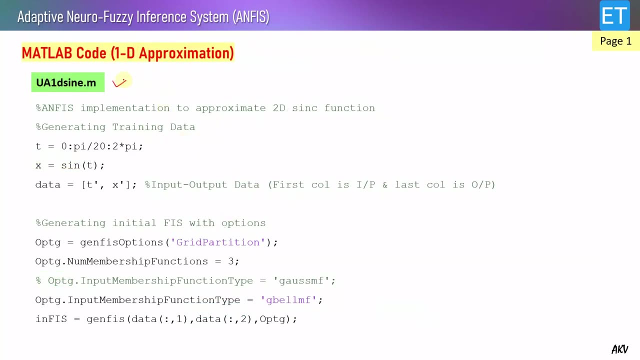 the two functions gen phase and and phase. gen phase is used to create the N phase model, While and phase is utilized to train that or Tune that. okay, so now let me come to the code. so this is the first file, which is for 1D approximation. I'm in sinc function, so first I'm generating the data. so this is: 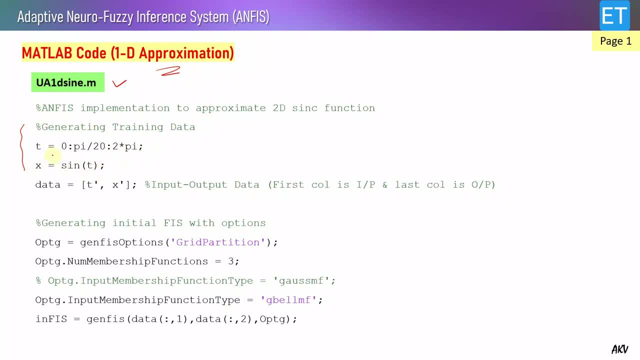 my t and this is the sin. so P is the x-axis value and x is y-axis value. so this is my sinc function for the religion sign, one cycle, and in the data i have arranged this t and x like this, so as a column vector i: 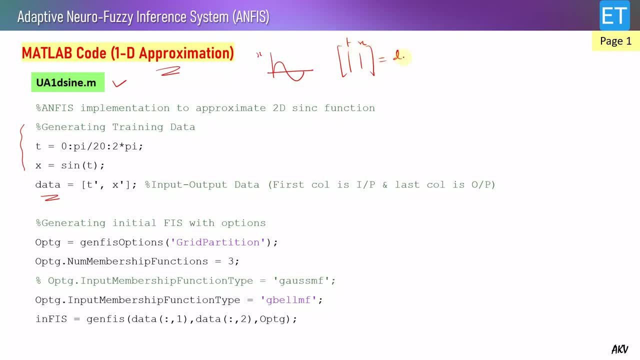 have arranged. so this is t and this is x in data right. so that will be used for training. now generating the initial fis. so with help of the gen face i will create my uh and face model. so first i have to uh, define some parameters, so we have the function gen face. 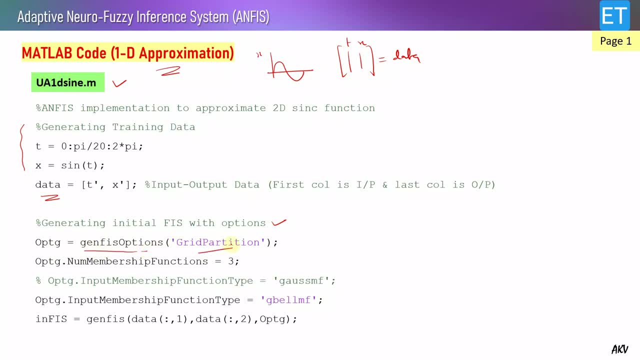 of options. okay, so i'm using the grid partition method. uh, there are other partition methods also, so if you go to the theory as proposed by the jank, you will have the better idea about what is grid partition. so, with help of the grid partition, i have created this option variable. 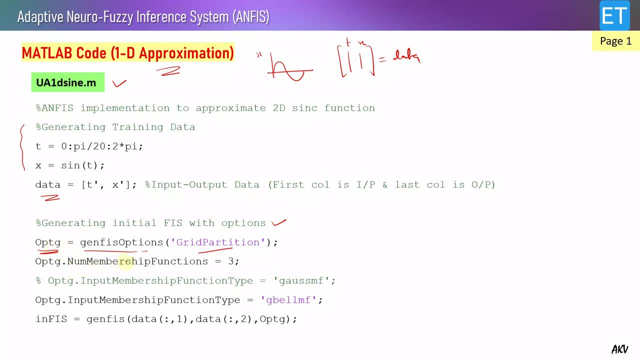 opt g. so now i will define the sum parameters, like how many membership functions i need. default is two, so, but here i have taken three, so optg dot. this is actually the matlab syntax you have to write as it is without any change. so number of membership functions: three. then opt g dot. input membership function type. 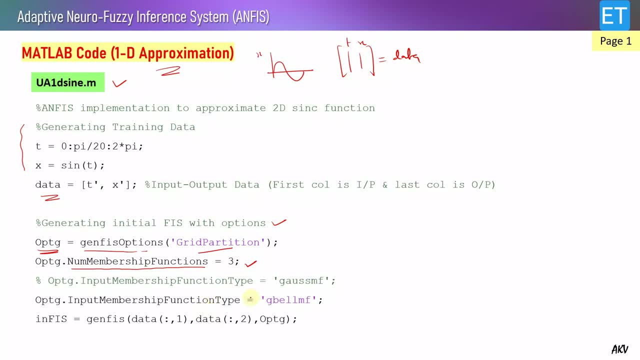 i mean which type of membership functions you- uh, you- are taking, so you can take any. there is a list in the matlab so you can take help of the matlab documentation here i'm taking the generalized bell membership functions. you can take a gaussian mf also. okay, so now with 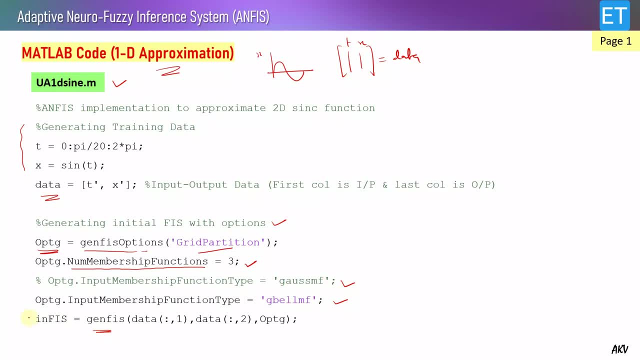 help of gen fish, i'm creating my model, my neural land, which has the name in face: uh, here you have to give the input, so this is the first column. uh, that is input and this is the output. so it will be treated as input and this will be treated as output for the network. so i have input output data. 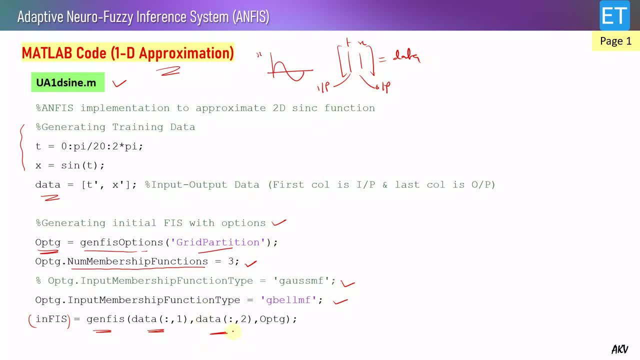 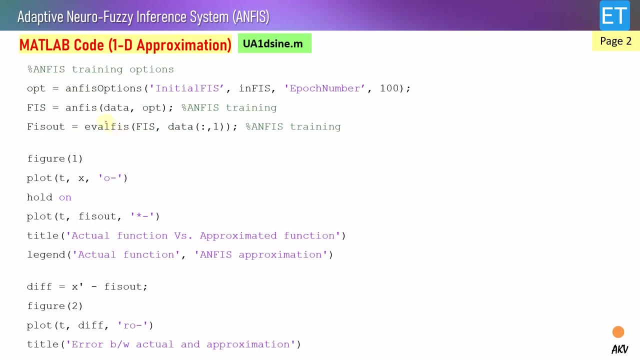 set available for training. okay, so with help of these options, uh, my network will be created with help of gen face, and this is my input and corresponding output. so now i will train this created model. so again, uh, you have some options, uh, that you can define during. 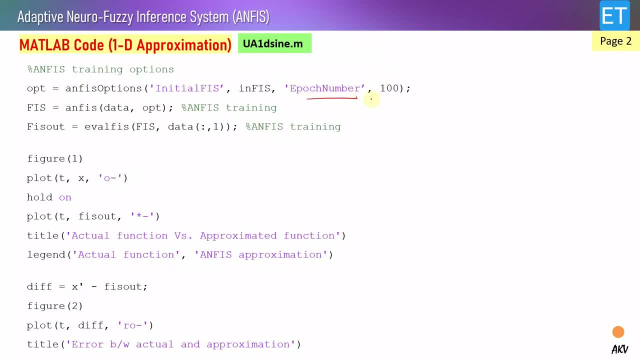 the training, for example, epoch numbers. i mean how many epochs you want to train. so here i am giving 100, the default is 30 and initial fis is in fis. so this is the model which is already created using genfis. so these are nfis options. so these are. this is the variable which is carrying all this. 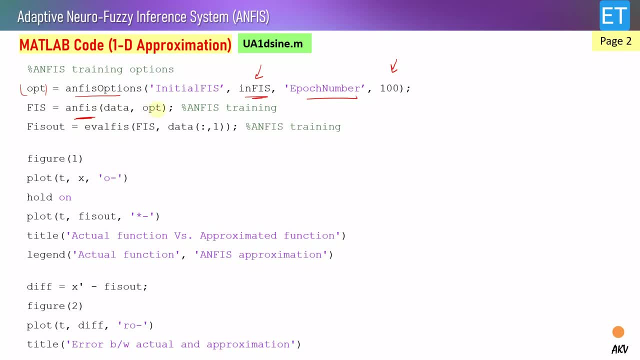 information opt. so now this is the uh function and phase which will train my model. okay, so nfis training is there. so with help of the options defined here, uh, with the help of the data which is carrying both input and output, the training is started and after the training, the complete model goes into this variable fis. so now fis training is. 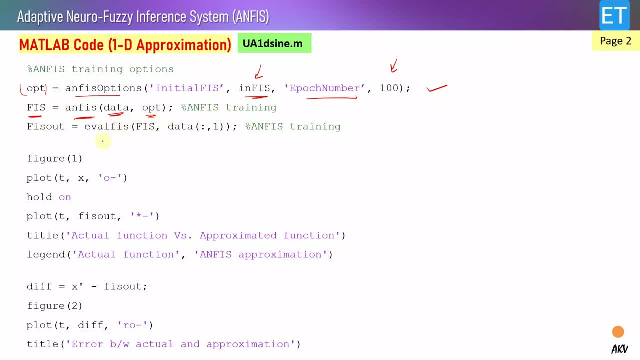 uh i mean and phase training is complete, then now you can evaluate it. so with eval face function you can uh find its output for any input. so i am giving the same input which is uh taken during the training uh data. i mean the second uh first column, that is a t column uh in this fis. so you 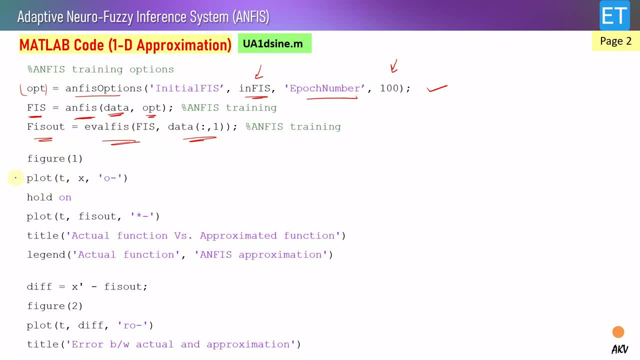 will get the output. okay. so now i am plotting uh the output. so first i am plotting the actual uh uh signal t versus x and then i am plotting this output. that is approximation done by the n-phase. so we can compare. and here i am finding the error. i mean, i'm uh finding difference between. 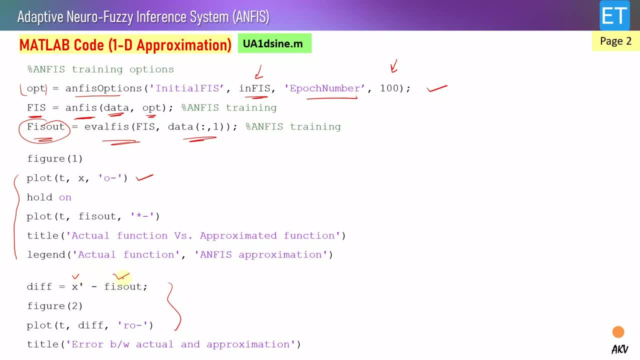 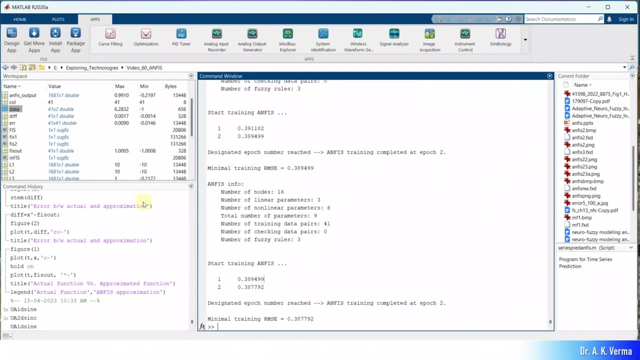 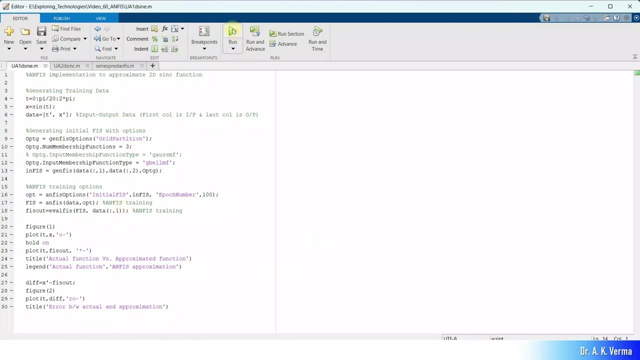 the original uh sine wave and the approximated sine wave by the n-phase, so we can see the difference. so let me uh jump to the matlab where i can show you the output of this program. so this is the matlab and this program is already written here. so let me run this program. 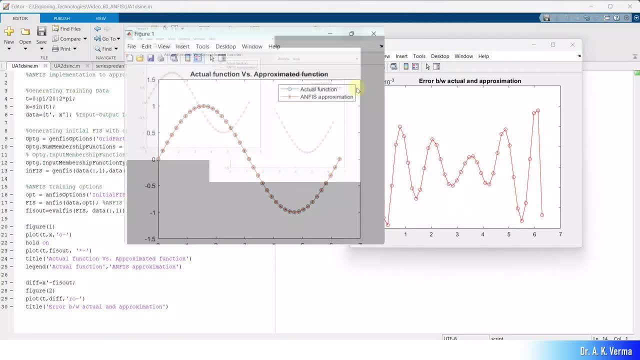 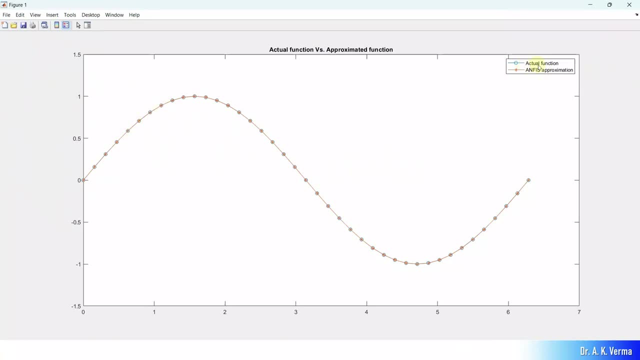 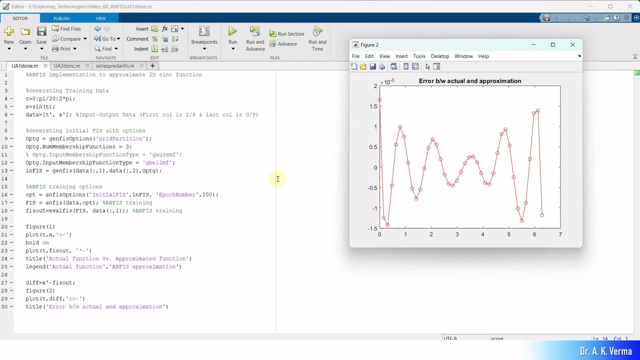 okay, so this is the output. so here you have actually the two curves, red and blue. so actual function is the blue and the n-phase approximated mission is given by the red. so here you are seeing a single one, but actually they are overlapping with each other. so, uh, here i'm taking the 100 epochs. 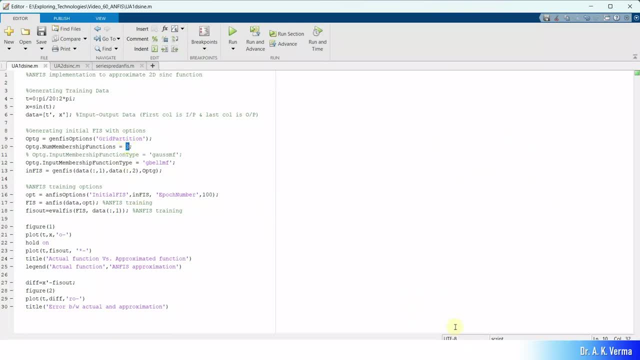 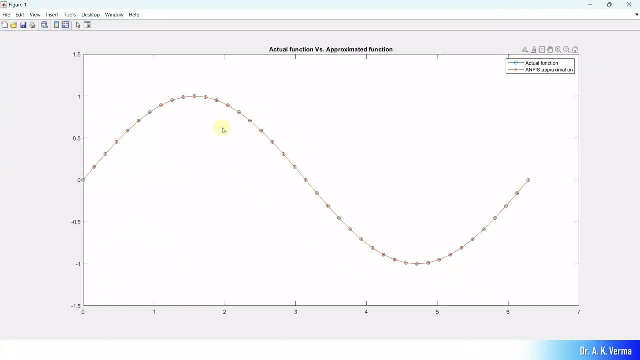 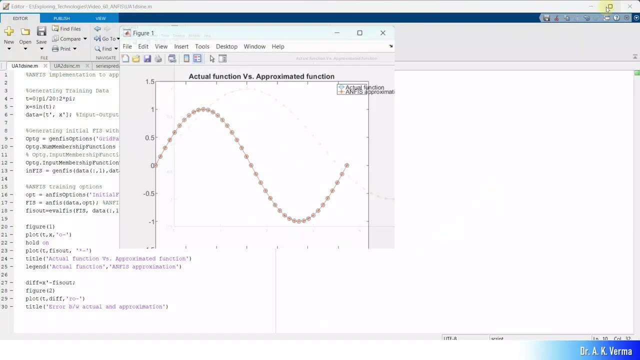 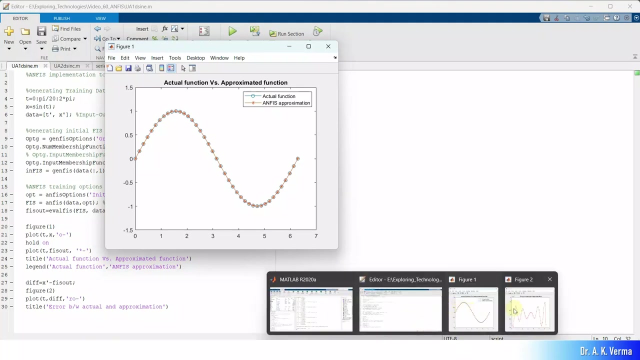 and three membership functions, so i'm getting very good approximation here. okay, so both are coinciding with each other. i mean actual function sign and the sign which is approximated by the n-phase. uh, by just looking this you can see that both are same, but exactly they. they are not same. there is some error if you subtract these two curves and 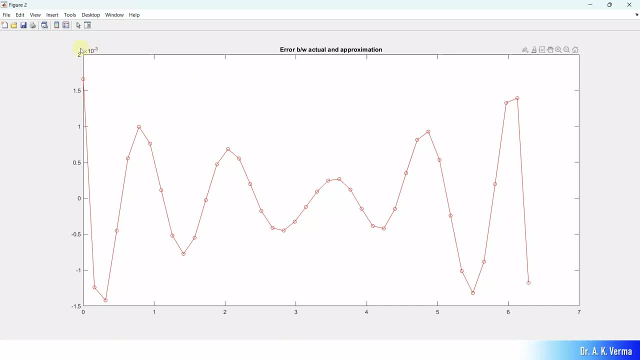 that is the error. so error is obviously in milli. you can see that 2 into 10 power minus 3, so some 10 power minus 3 values. so you can see that both the curves are very, very close to each other. so that is a very good example of that. how close. 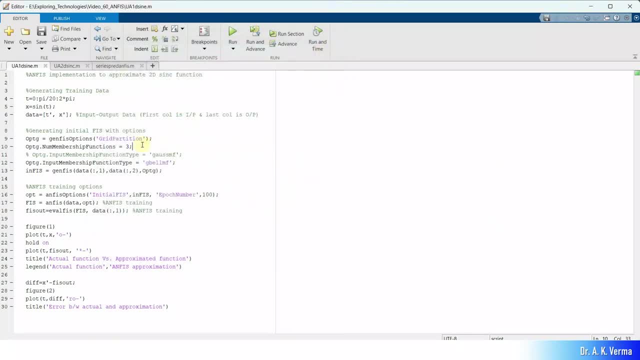 is approximation, but you can see the difference. so instead of let's say membership function 3, i can make it 2, and the epochs, let me take it 30. so i have reduced the number of training epochs to 30 and the membership functions per input is 2.. 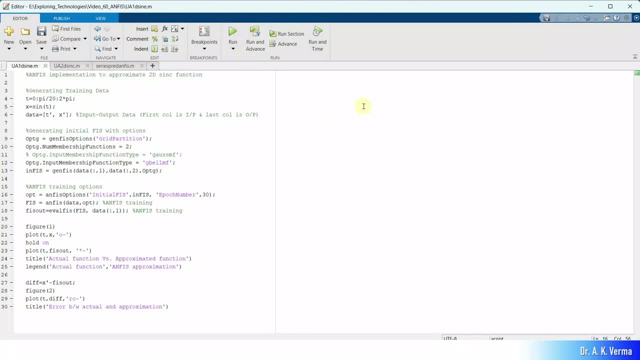 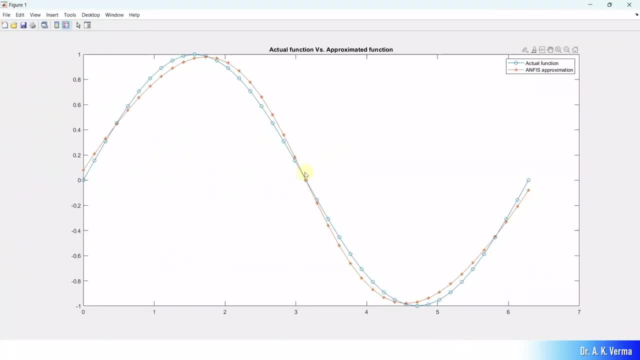 so let me run this program and see what is the difference. okay, so this is the error. and now, here you can see the difference. so this blue one is actual sine wave, while this red one is a approximated sine wave, i mean the approximation done by the n-phase. so n-phase has trained itself. 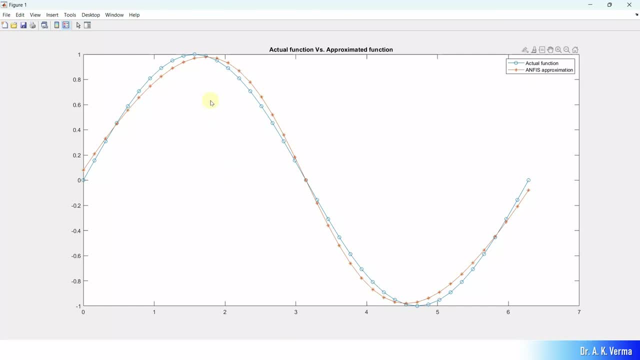 you understand, n-phase has trained itself. so for any input t, it will give the corresponding red output, although it should get the blue. it should give give me the blue output, but it will give me the red output with the difference. so at every instant you can see there is some difference. 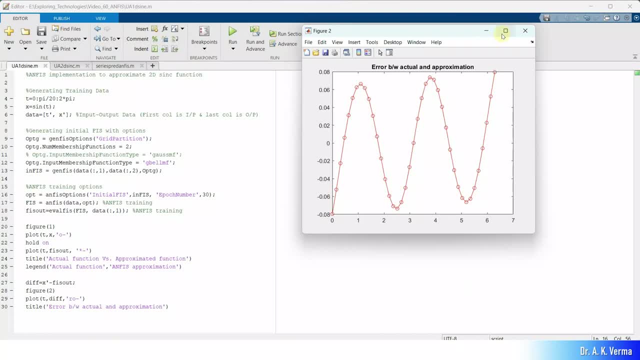 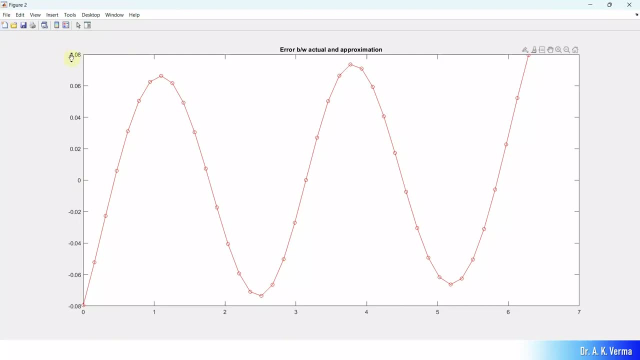 and difference is huge now. so with help of this error, you can see at the different instant of time. we are getting error up to the 0.08, although it is very small. but as compared to the previous case where the error was in the milli 10 power minus 3, this is. 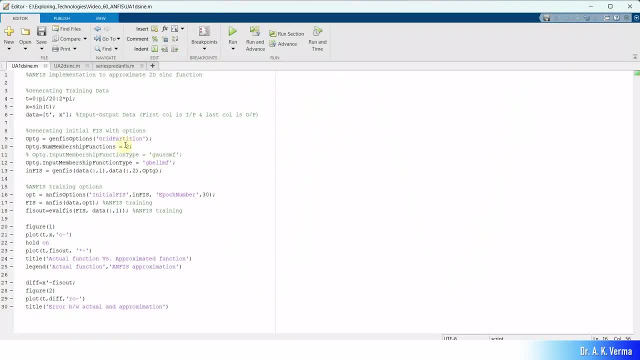 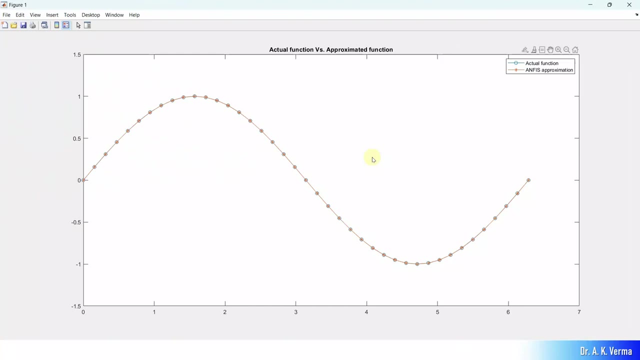 not good. so just by increasing the membership function uh to the three and the uh epochs number to the hundred, i'm getting very good approximation. so that is the output. so here the both the curves are coinciding with each other. so i can say that my end phase is now behaving as 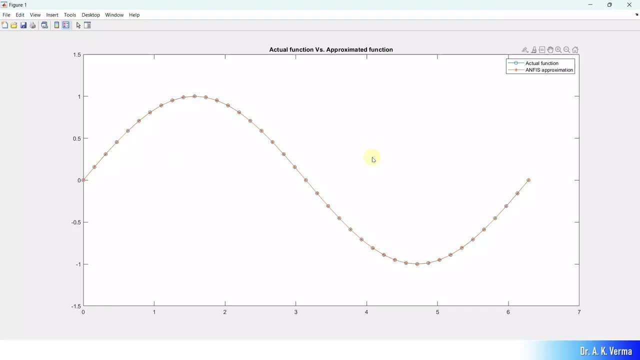 a sine function. so whatever input i will give, uh to the n phase. it will simply take a sign of that and give you the output. so my n phase box, you can say that model or that system is behaving like a sine function. so it means uh, uh with by appropriately choosing number of membership. 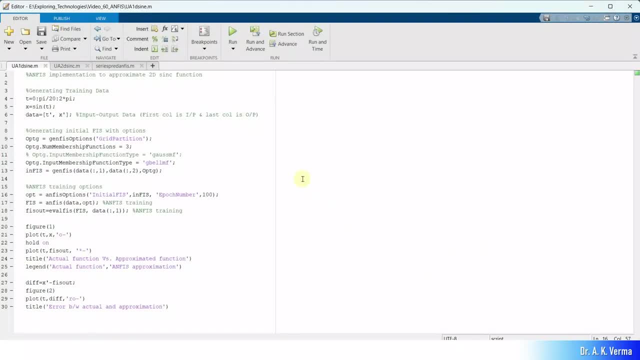 functions and uh number of membership functions. i can take that number of membership functions and the number of number of training epochs. i can make my end face to behave like any one dimensional mathematical function. so that is that's why i call it as a universal approximator, right. 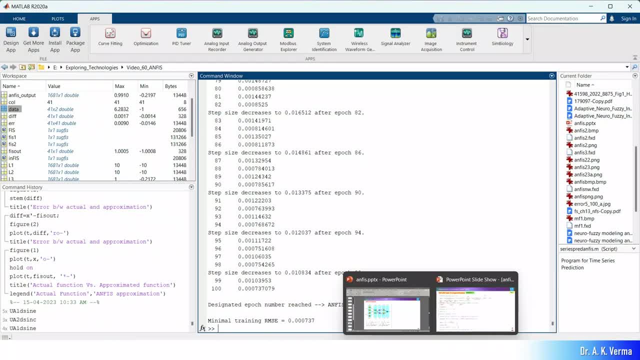 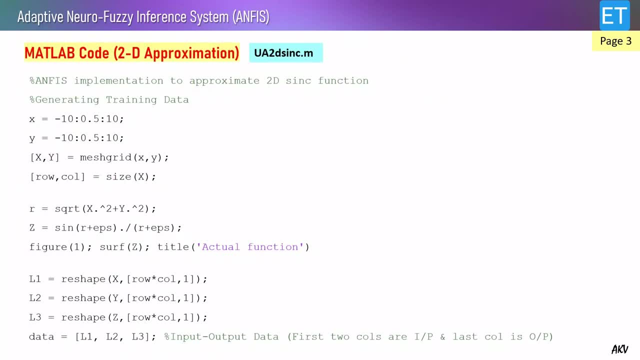 so now let me uh jump to my presentation back, and here i will take the example of the two dimensional approximation. so in the previous case i have taken, uh, the one dimensional sine function. now i will show you you can approximate a two dimensional function also. that is really complex. 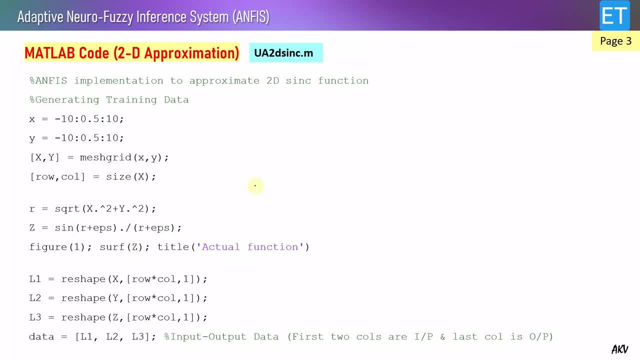 i have already shown you that i have taken the case of the two dimensional sinc function. so i am defining the variable x and y, then match grid- both x and y are ranging from minus 10 to plus 10- and then square root of x square and y square and this is my sinc function. 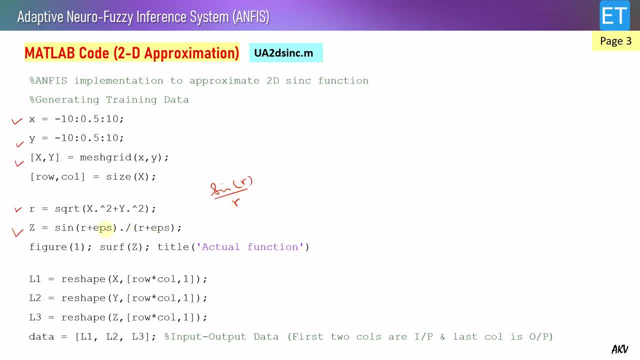 that is, sine r upon r. here eps is added just to avoid 0 upon 0, because when r is 0 then there will be sine 0 upon 0, 0 upon 0, so that will be undefined. so the eps will avoid this error. so i am plotting this: 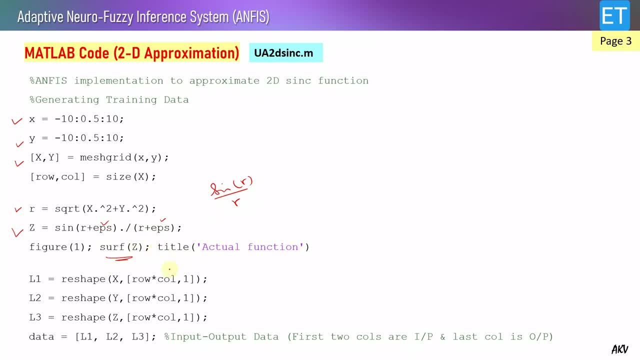 actual function with help of the surf function, then i am preparing the data. so i have. just because these x and y are two dimensional, so i, uh, i have converted them into the columns, okay. so x is converted into l1, y is converted into l2, l1l2 and the output z is converted into l3. so z is converted into l3. 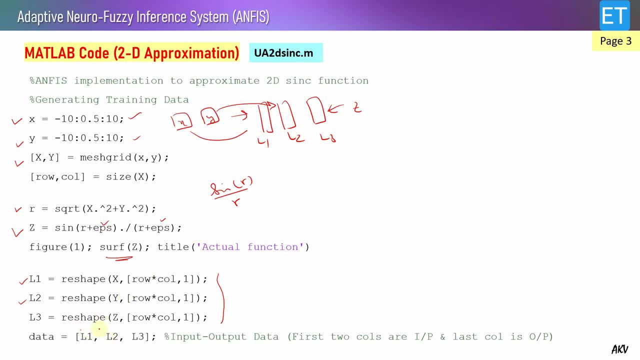 l1, l2, l3, all are uh, combined together here to make the data okay. so data variable is created which is carrying all the inputs and output. so in this matrix, the first column is l1, which is carrying the x, the second column l2, which is carrying the y, x, y, input, and then z. the third column is z. so 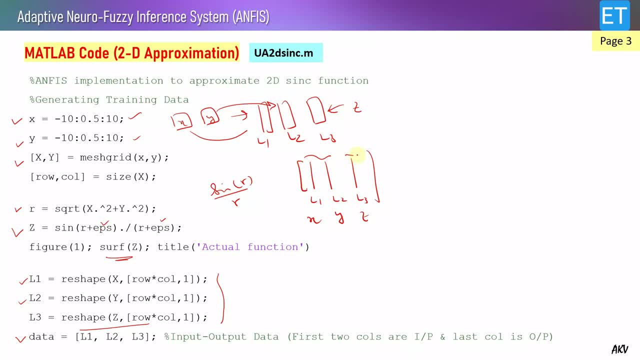 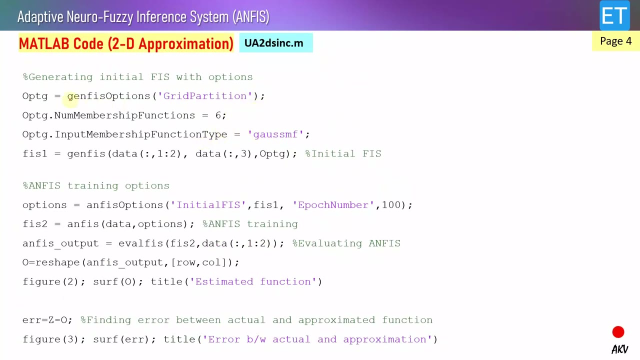 these two first two columns are input, while this last column is the output. so all input outputs are arranged in this data matrix. and now again the same type of syntax which we have already seen in the previous uh example. so first, with help of the gen fish, we will create 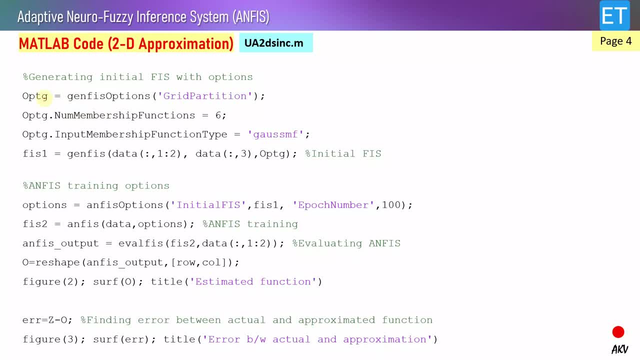 the structure and first, but before that, we have to define its parameters. so with help of the gen face options, we will define the number of membership functions- we are taking six per input- and then we are defining the input membership function type. so here we are taking gaussian. 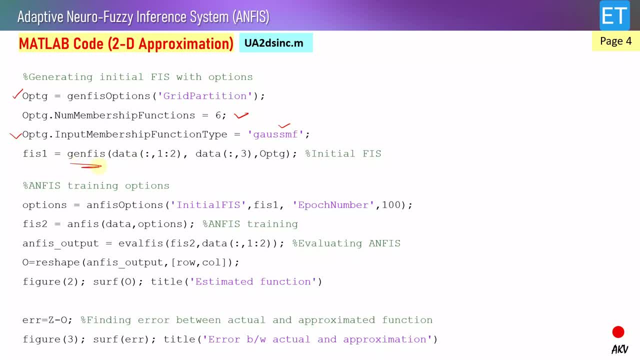 membership functions. then with help of gen face, we are creating this model, fis1. so here, this is input- i'm in the first two columns, uh, x and y, and this is output z and then options defined here. so with this gen face option, the fis1 model is created. now, uh, the end phase. 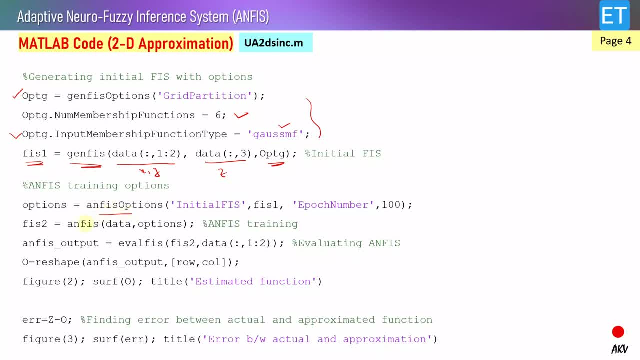 option: uh, we will train the model. so this fis1 is here. initial fis and epoch number is 100, so iterations will be uh done in the 100 epochs. you can change it as per your requirement. and now, with and face, we are starting the training with all inputs and outputs and then options uh given in this line. so 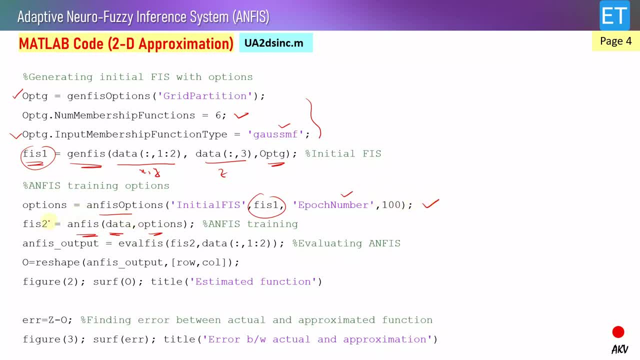 once the training is done, we will start the training. it will take time, uh, uh, because it is uh, more, more complex, because we are taking six membership functions and 100 epochs right. so, uh, once the training is finished, uh, this fis2 is my trained model, so it should behave like that two dimensional sync function. so for that we have to. 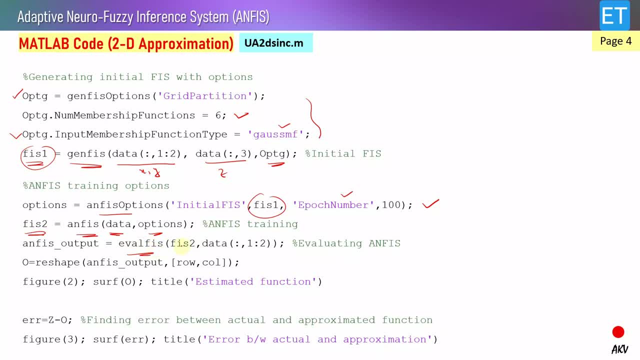 evaluate it. so with eval phase we have given the input x and y to this model and the corresponding output is this. so emphasis output is my approximated output, right? so since it is in column matrix, so I have to convert back into the two dimension. so with the 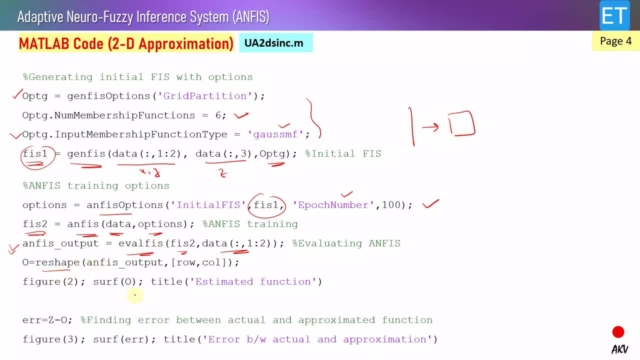 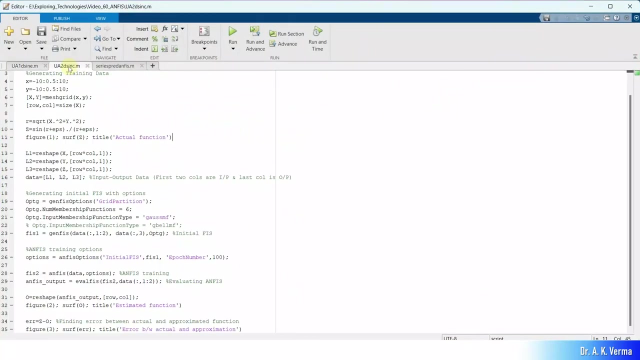 help of the reshape I am converting back into the two dimensions and then I am plotting it with a surf, and here I am finding the error between the actual and the approximated plots. so now I will show this into the MATLAB and then we can have idea how it is working. so this file is is already written here, so let 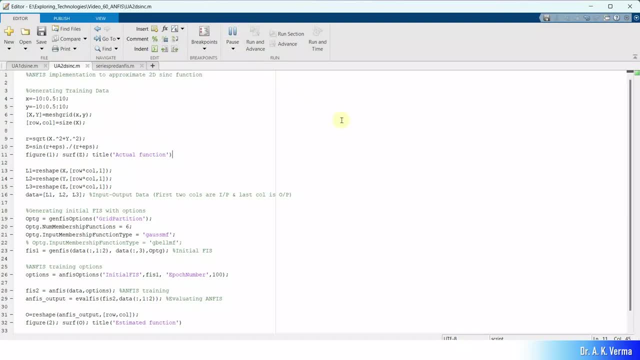 me run this. it will take some time because the system is now more complex and we have defined a hundred epochs. so, depending on the speed of your complex, you can find the error between the two dimensions. so I am going to compute it. it will take time. so let me see what is happening in. okay it, yeah, it. 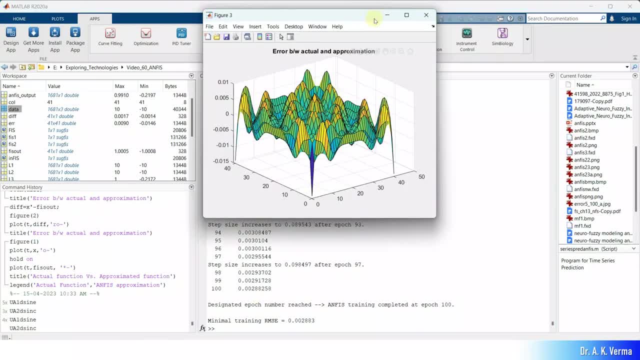 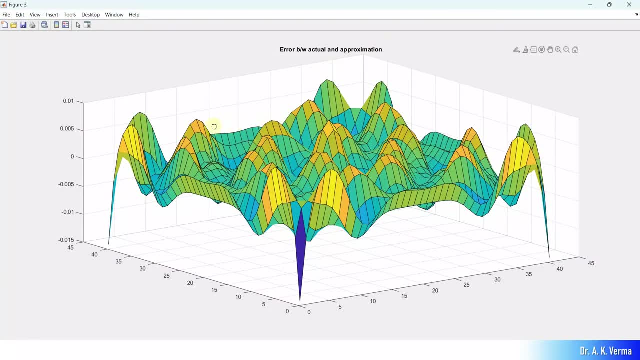 is still busy. MATLAB is still busy. yes, it is done. so this is actually error between the actual and approximation. so you can see this is the error and it is going up to the zero point, zero one that is also in milli, 10 power minus 3. so I 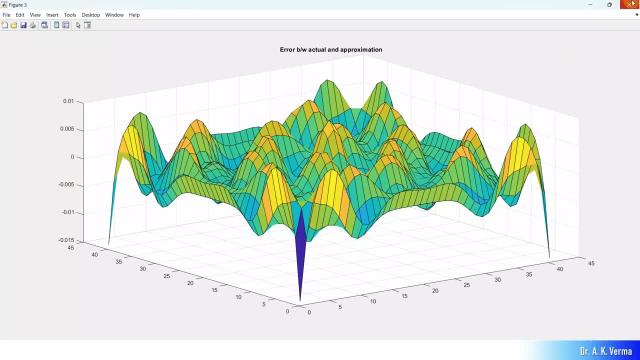 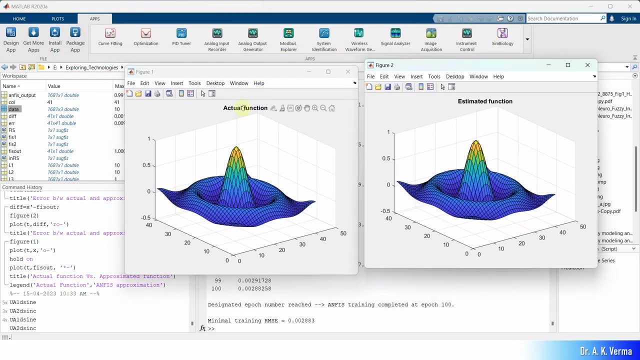 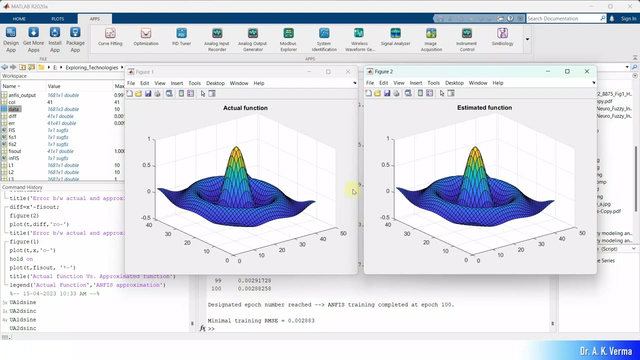 should expect a good approximation in this case. yeah, I get that, get this. this is actual function and this is the estimated function you can see. so both look very similar, but of course there is a difference, as we had just seen in the error plot, but they look very similar. okay, so this is your. 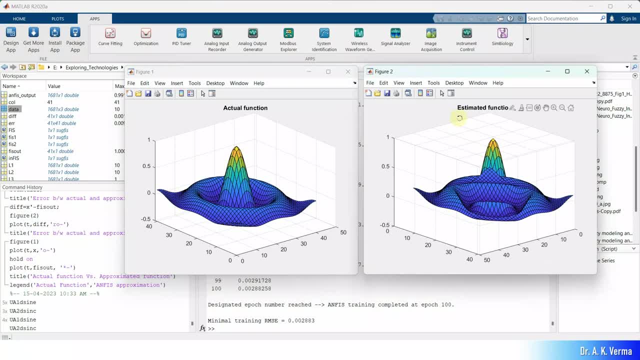 actual sinc function and this is approximated sinc function. so now you can say that my end face model is trained and it is behaving like a two-dimensional sinc function. so if you give any input of X and Y, it will create the Z output. okay, and that is equivalent to the finding sinc of input values X. 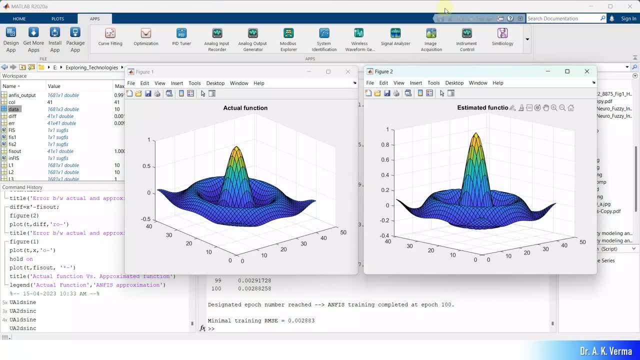 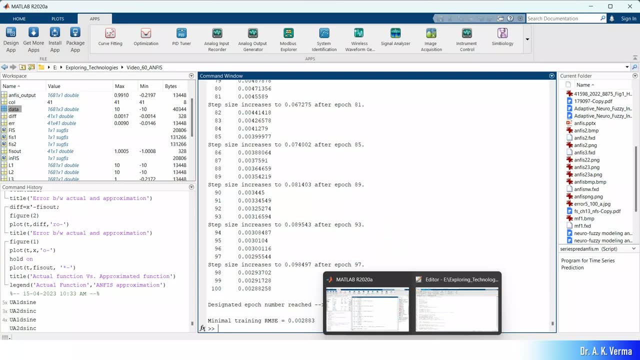 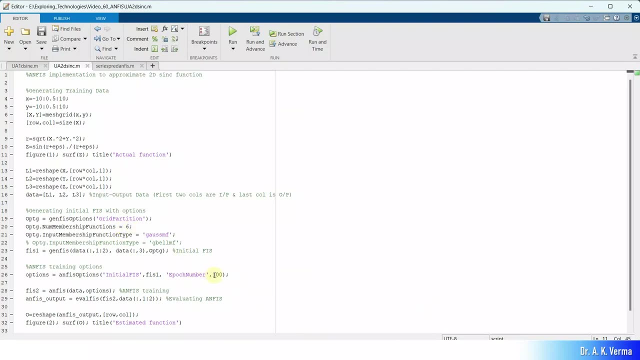 and Y. so this is one good example. now let me show you the some differences in the input and output. this is the best and I will not say best, but this is a quite good approximation, because I have taken the six membership functions and hundred epochs. so let me reduce the number of a epochs. let's say epochs are. 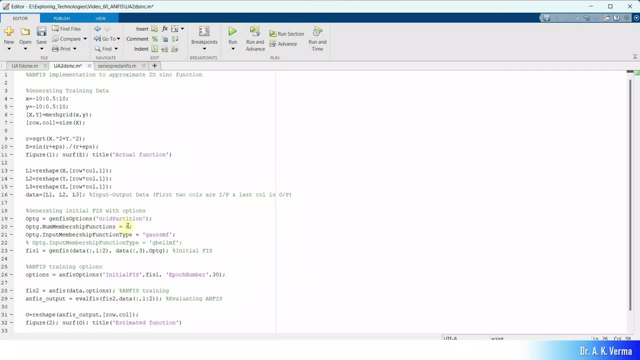 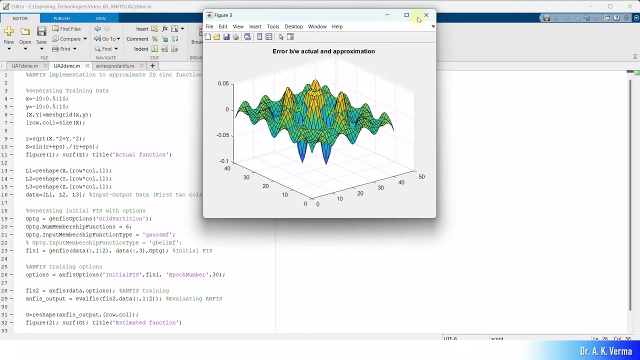 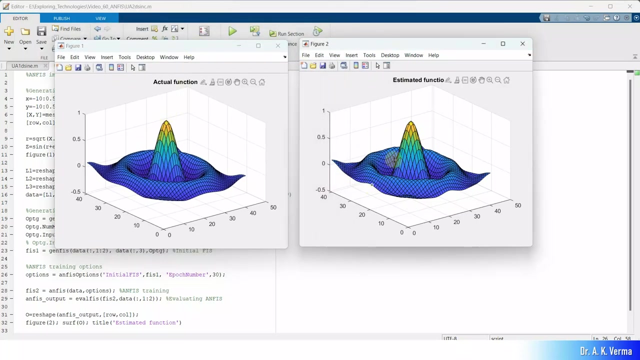 30 and the number of membership functions are: let me let let it remains 6.. so run this program and see what happens. okay, so this is the error and thank you for fanning this video. estimated output and this is input. so it is not good, actually, from upside it is. 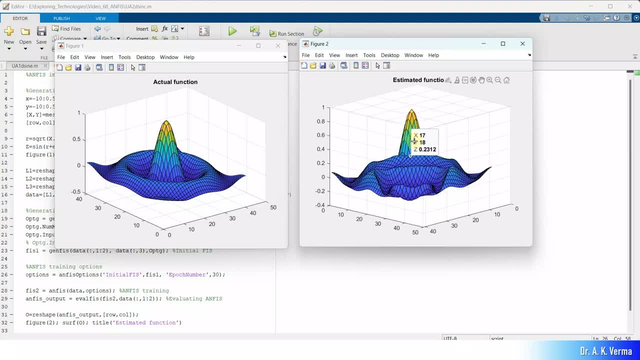 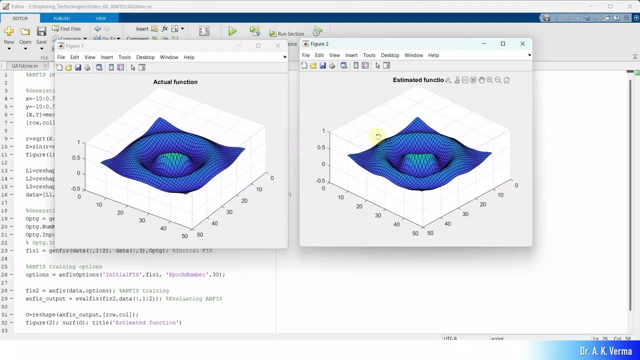 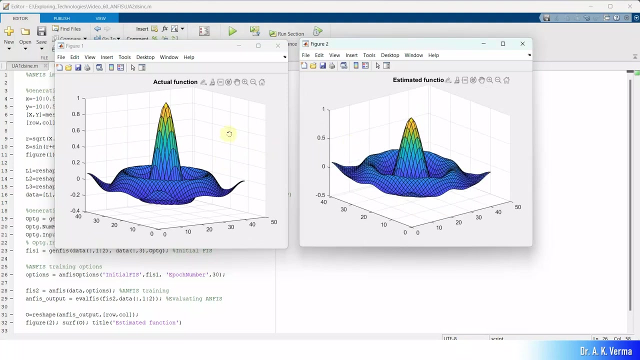 looking almost similar, but if you see the downside there is a difference. here you can see a perfect circle in the bottom, but here it is not a perfect circle. I am getting some bounces here right, some ups and downs like this, so there is a huge error actually as compared to the previous case, when I 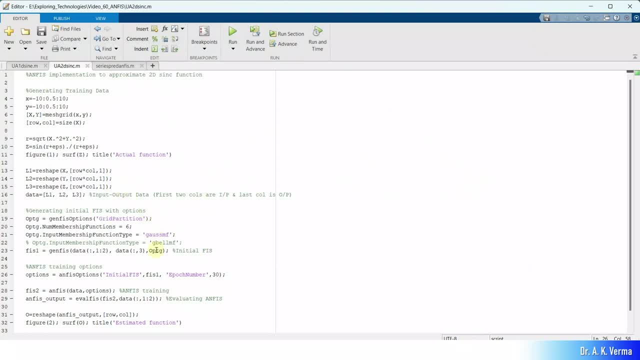 reduce the epoch numbers. so now let me take one more example where I will reduce the number of membership functions. so I keep membership functions free and epics to be. let's save 50 and let's see what will happen. okay, so this is the error and this is. 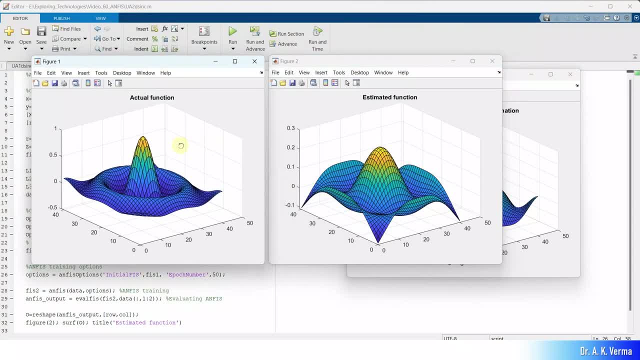 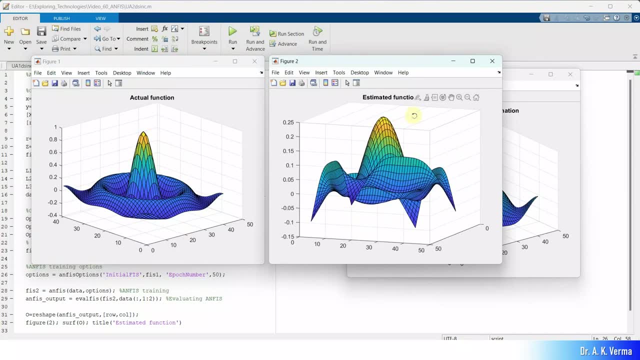 advantage. this is your applications. so if you consider this here, moment, initially, okay, so this is the error and this is the error, and this is the activity and estimated and this is actual function, so you can see that there is a huge difference. so this is my actual function and this is the estimated function or approximation. so this is not matching at all. 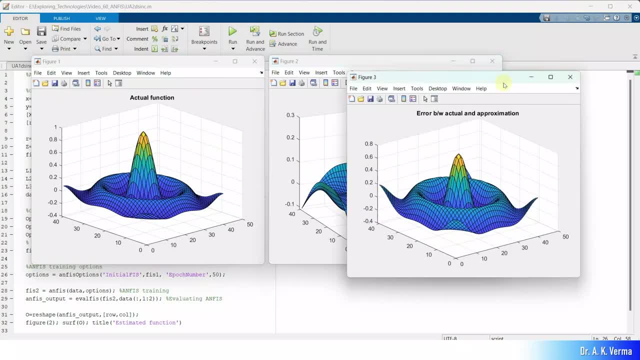 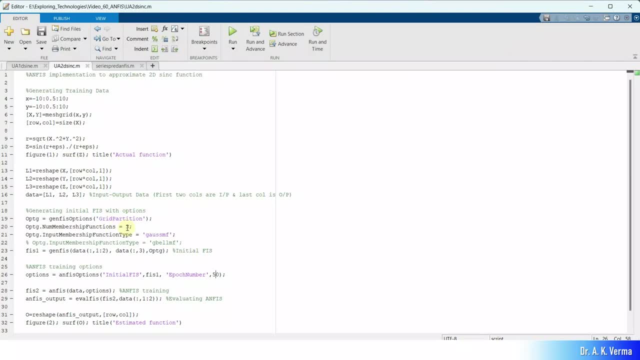 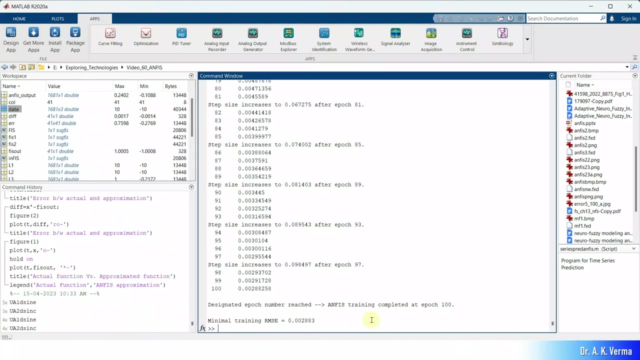 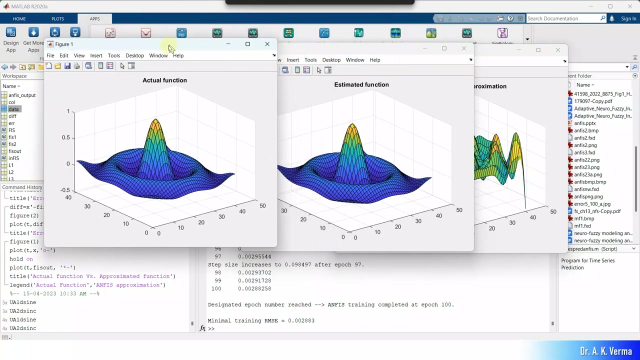 with this input function, as you can see that there is a huge error. so obviously, by reducing the number of membership function, it is working very badly. so let me go back to the six and epochs to 100, so it is giving me the quite good approximation. okay, so this is, uh the case where i have taken six membership functions and the hundred epochs. 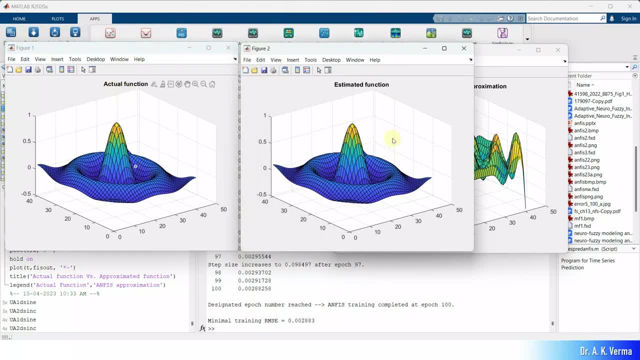 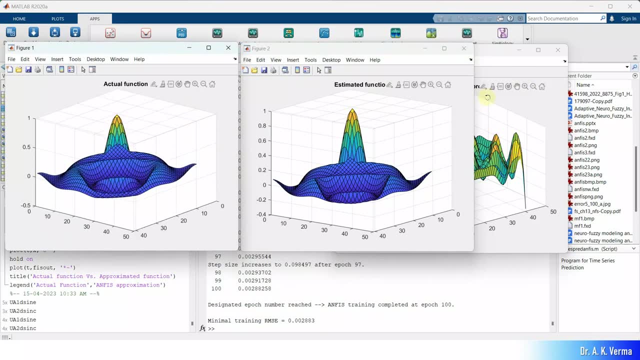 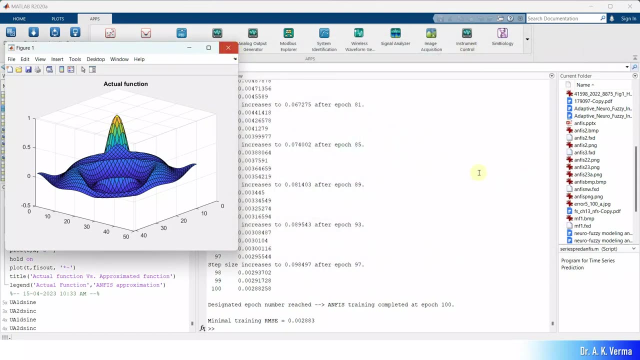 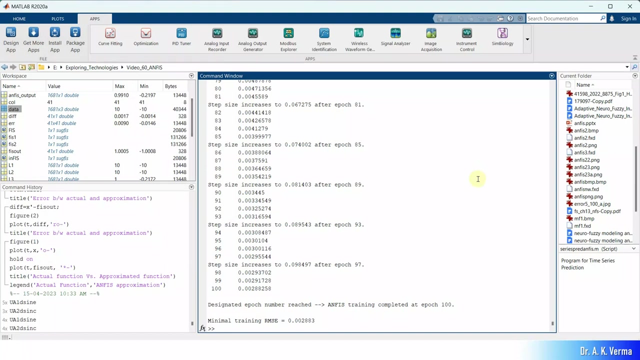 so this is actual function and this is the estimated function you can see. okay, so that is giving me quite good approximation, with very small error like 0.01. so this is, uh, how an and phase model can be trained to approximate any mathematical expression. so that's why we say it as universal approximator. 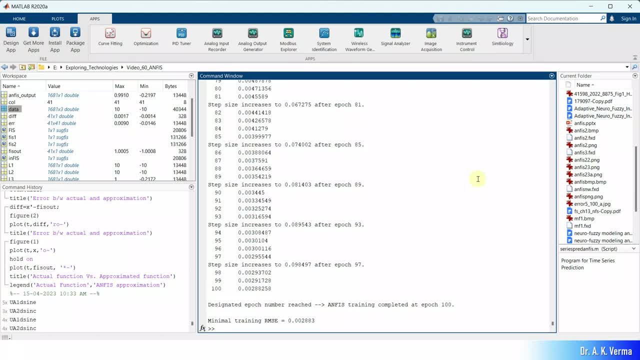 so, in similar way, you can train any and phase to work like any mathematical functions. i mean, you can design some controllers also, because controllers are also some mathematical equations, right? so, okay, that's it for this video. i hope you have liked it and you have learned something new.